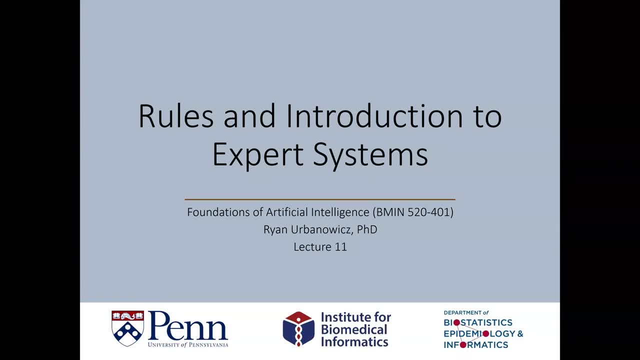 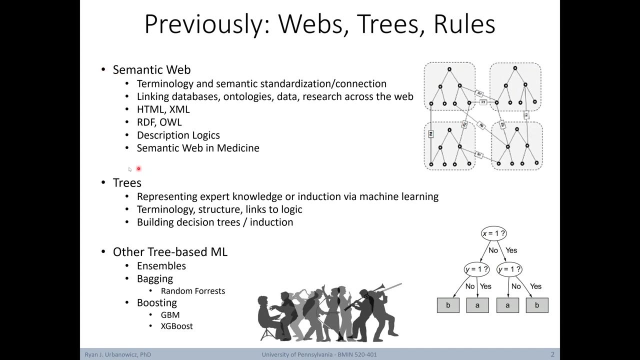 Hello and welcome to lecture 11 of Foundations of Artificial Intelligence. Today we're going to learn about one other form of knowledge representation, in particular that of rules, and then this will segue into an introduction to expert systems. In our last lecture we covered semantic webs. we learned about trees as another form of knowledge representation. 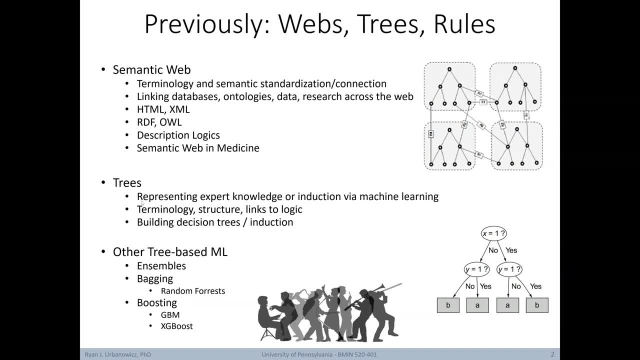 and also learned about decision trees as an induction method for machine learning. And, lastly, we gave a tour of other machine learning algorithms that are based on decision trees. In particular, we learned a little about ensembles, bagging and boosting. 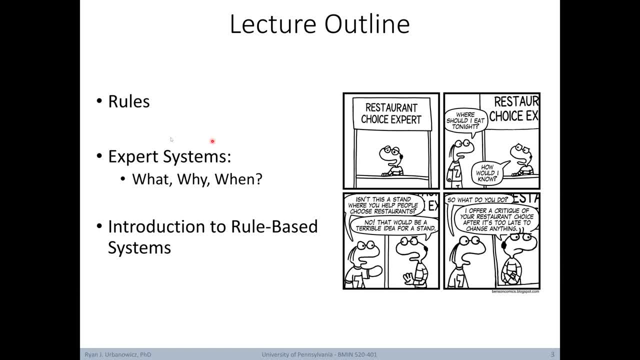 Here's the outline for today's lecture. Again, we're going to cover rules, expert systems, including what they are, why they're useful and when they're a relevant choice to either build or use. Then, as a precursor to our next lecture, we'll give a brief introduction to rule-based 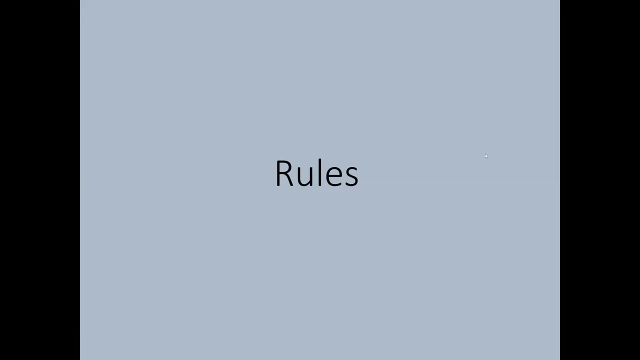 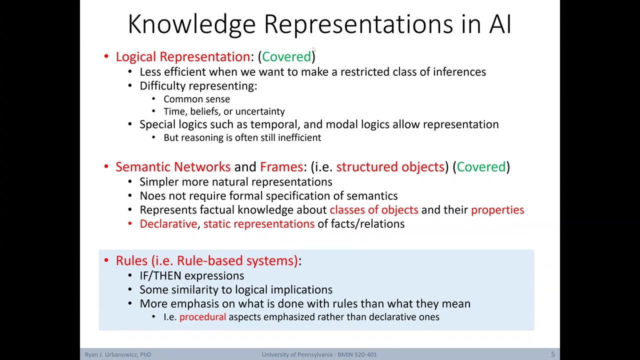 systems, which is a particular type of expert system. We begin by looking at rules as an another form of knowledge representation. We've seen this slide in an earlier lecture that laid out the key knowledge representations that we're going to focus on in this course. 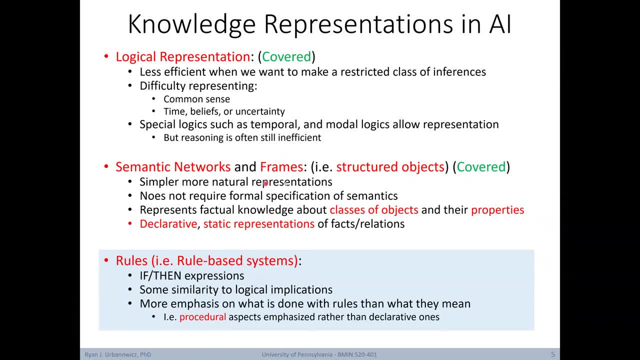 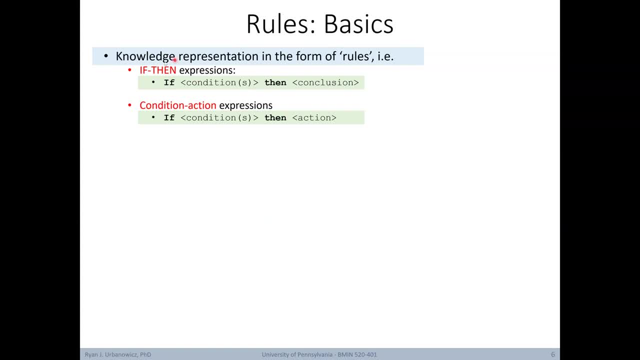 The first were logical representations. later we learned about semantic networks and frames. and finally, today we're going to talk about rules. Rules are pretty straightforward. They're typically given as if-then expressions. You have, if one or more conditions, then some conclusion. They can similarly be represented as condition-action expressions. 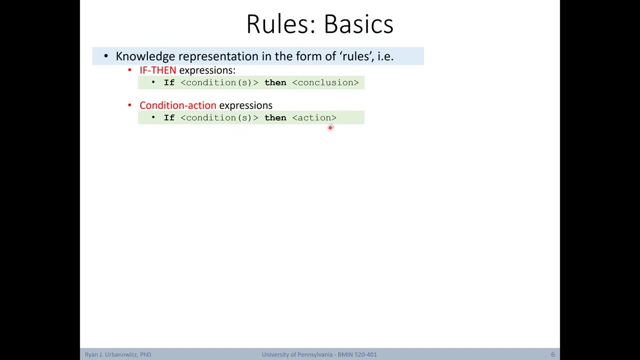 So again, if one or more conditions then do some action, Rules themselves are effectively propositional or first-order logic implications. Here's a really simple example of a rule: If the traffic light is red and you have stopped, then a right turn is okay. A quick biomedical example. 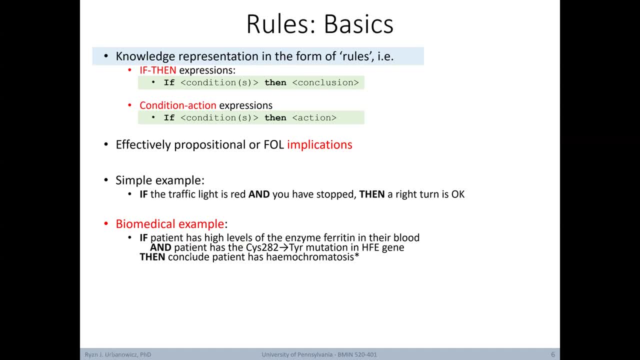 if patient has high levels of the enzyme ferritin in their blood and patient has the cis-282 thyroxinase mutation in HFE gene and patient has the cis-282 thyroxinase mutation in HFE gene, then conclude: patient has hemochromatosis. The first two conditions, given the if statements. 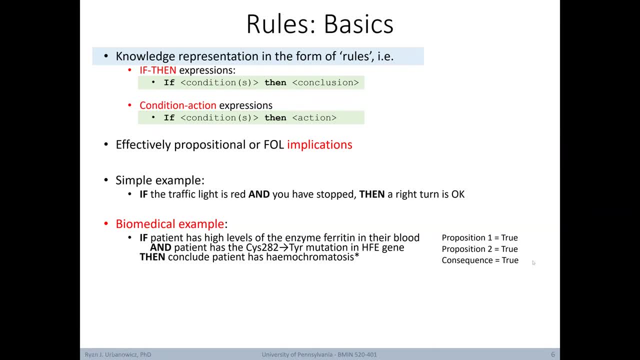 are separate propositions which, if true, indicate that our consequence or conclusion is true. The term condition is also known as the premise, the antecedent, or you can think of them as independent variables. The conclusion can also be referred to as the action, the result. 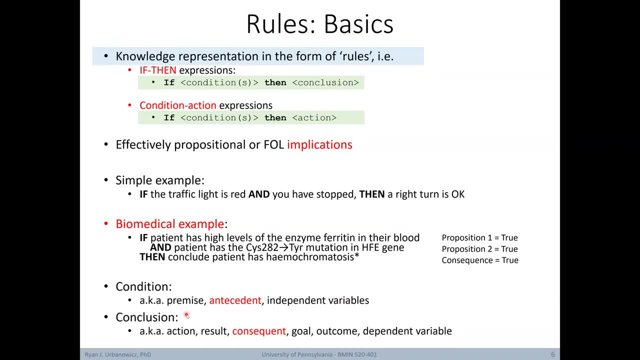 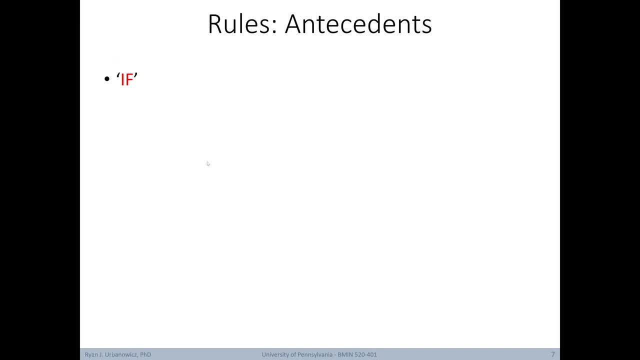 the consequent, the goal, the outcome, or you can think of it as a dependent variable. Let's dig a little more into the rules. antecedent or its condition. This is the if part of the rule and the antecedent represents a. 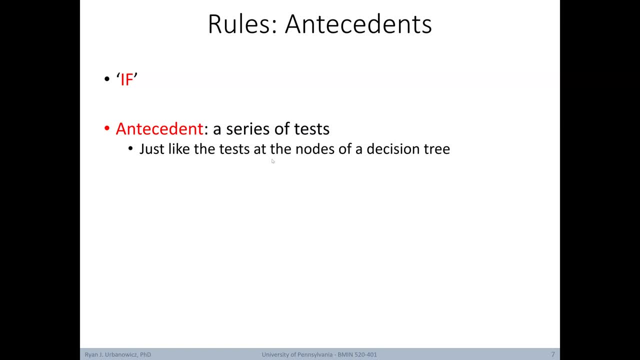 series of tests to be conducted, not unlike the tests at each node of a decision tree. There's some natural links between rules and trees that we will identify further later, but it's first worth noting that, in terms of expert systems, rules are a popular 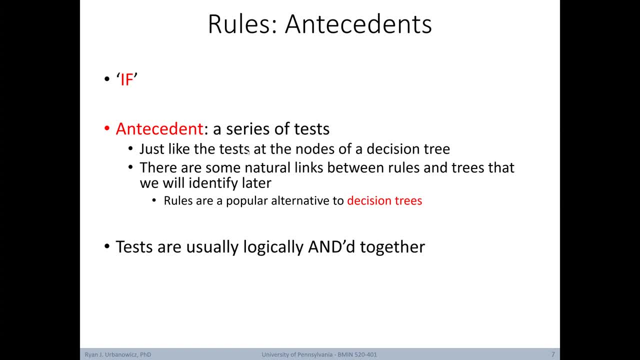 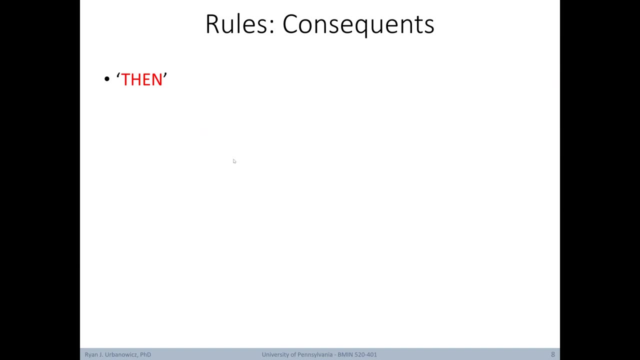 alternative to decision trees. These tests that make up the antecedents are usually logically AND together. This is similar to the definite clauses from logic used for chaining and inference. However, in certain circumstances, rules can have different logical expressions in them. Now let's take a closer look at the conclusion, or the consequence of the rule. This is the then. 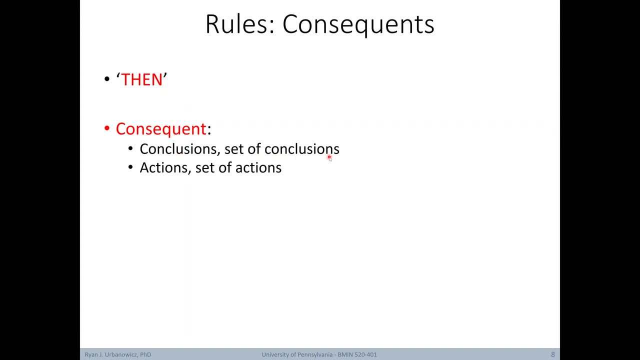 portion, and the consequent can either be a single conclusion or a set of conclusions. Similarly, it can be an action or a set of actions. Additionally, for each conclusion or action, the consequent can have a probability distribution assigned by the rule specifying the support or certainty. 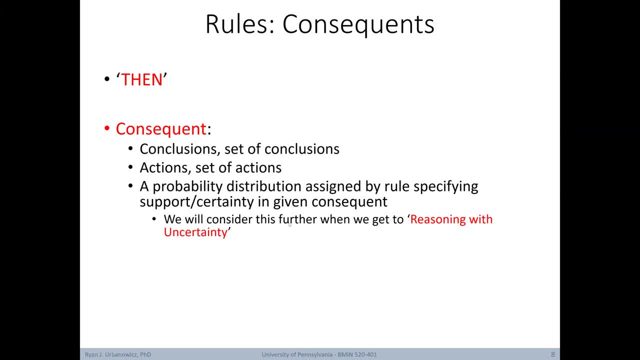 for that given consequent. Let's go further when we get into reasoning with uncertainty later on in a later lecture, It's good to note up front that if you have multiple rules whose antecedents are satisfied, then you can end up with a situation where you have conflicts in terms of the consequence. 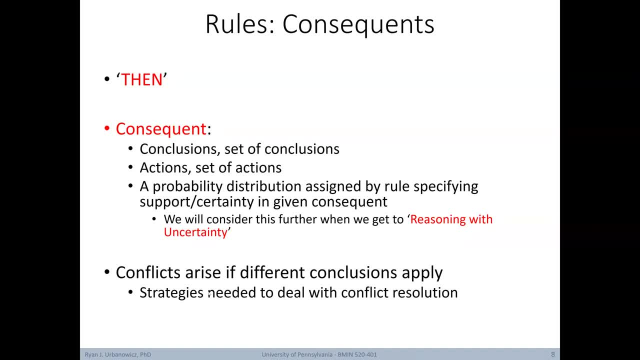 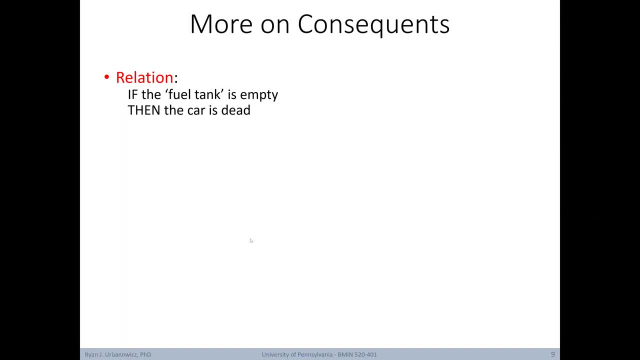 being asserted. So like from semantic networks, we can have situations where we need to deal with conflict resolution. Consequence can be used in a number of ways. One is to express a relationship. In other words, if the fuel tank is empty, then the car is dead. 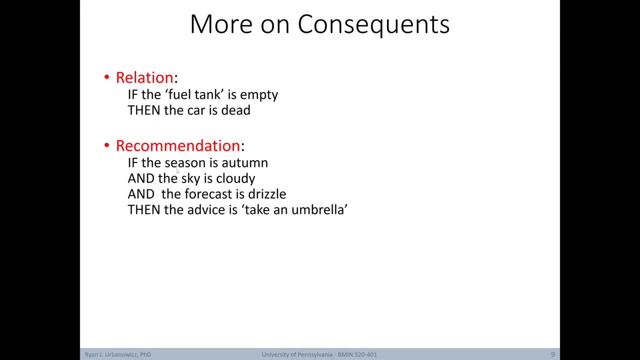 They could also be utilized to make recommendations. So, for example, if the season is autumn and the sky is cloudy and the forecast is drizzle, then the advice or recommendation is to take an umbrella. Consequence can also represent directives, or you can think of them again as actions. So in 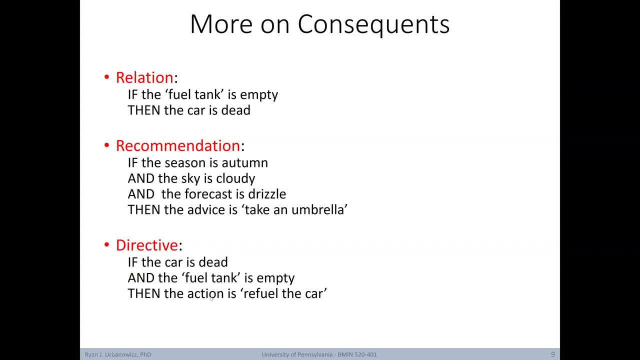 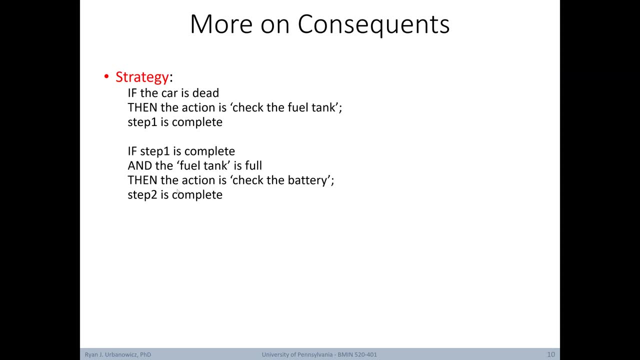 this case, if the car is dead and the fuel tank is empty, then the action is refuel the car. Further consequence can be used to set up some higher level strategy. As a rough example of this have: if the car is dead, then the action is check the fuel tank. Further, add the fact that step one 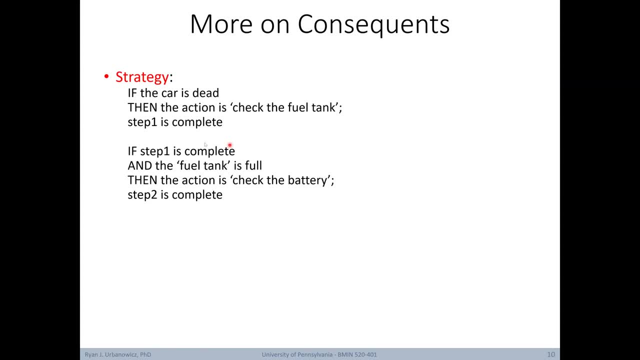 is complete, Then another rule in the knowledge base might say: if step one is complete and the fuel tank is full, then the action is check the battery And at this point the fact step two is complete will also be added to the knowledge base. And lastly, consequence can be used as heuristics. 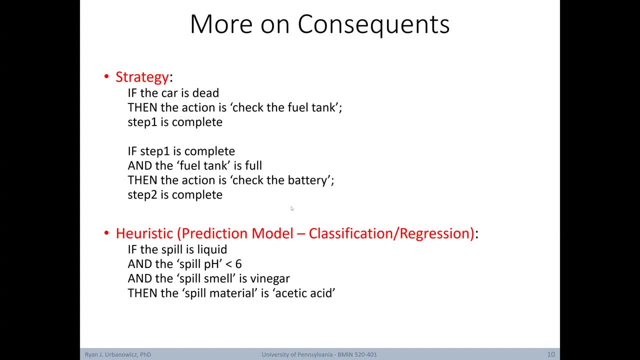 to represent some kind of prediction model, either for classification or for regression. As an example we have: if the spill is liquid and the spill pH is under six and the spill smell is vinegar, then the spill material is acetic acid. In this case we have some evidence that is being 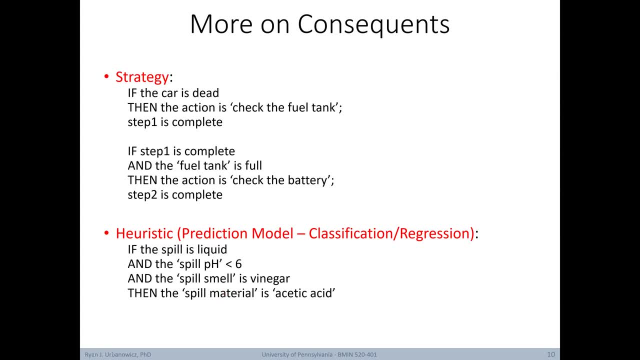 used to support some prediction as to what the outcome material is, Depending on the certainty of the facts as well as the certainty of the association between the facts and the outcome. this prediction here at the bottom in the consequence can have some certainty associated with it, going from 100% confidence to 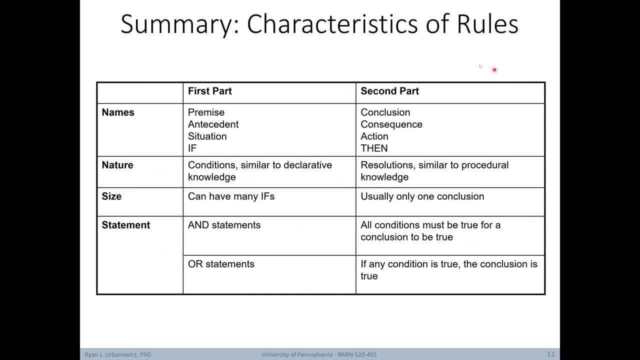 something much lower. Here's a summary of the basic information about rules for your reference in the future. It includes information about names that we just covered. the nature of these two parts of rules, where conditions are similar to declarative knowledge and consequence are: 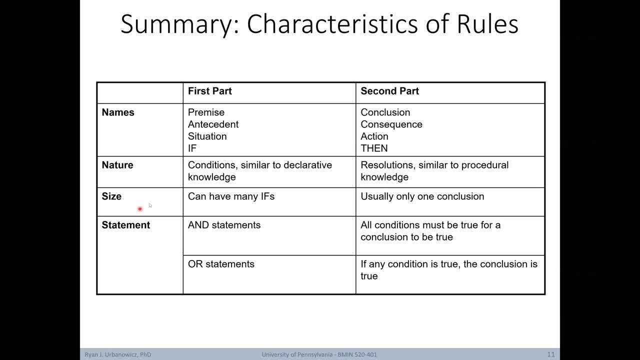 resolutions similar to procedural knowledge. In terms of the size of the parts, the antecedents can have many ifs linked by ands usually, And typically the consequence usually have only one conclusion, but this is not always the case. And then we have the two most 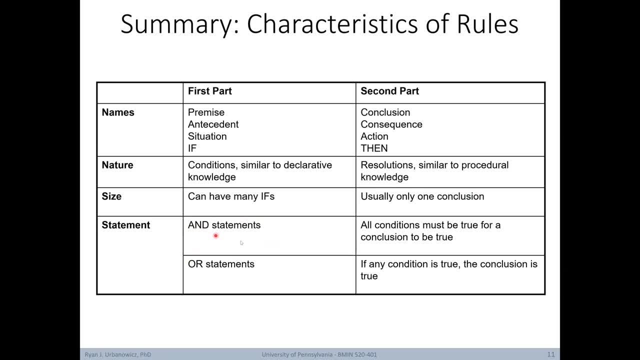 common kinds of connectors found in rules and or or where for ands. all conditions must be true for the conclusion to be true And obviously, if we have ors linking them, if any of those conditions is true, then the conclusion is true. We can also add a variety of conditional relations to rules. 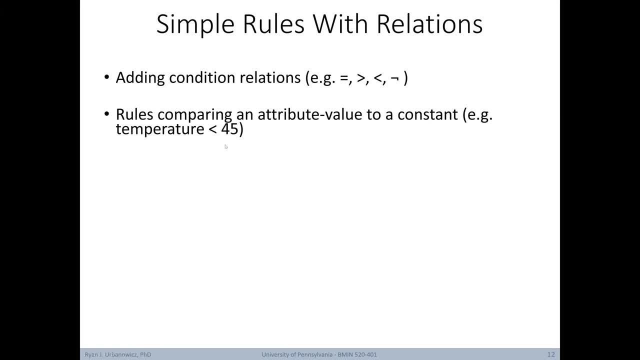 Rules can compare attribute values to a constant, for example temperature less than 45 degrees, And these would be called propositional rules, which have the same expressive power as in propositional logic. For example, if credit rating is high and salary is no more than 30000 pounds or assets are, 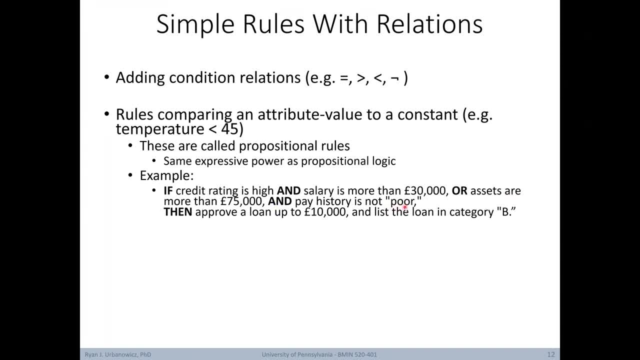 more than 75000 pounds And pay history is not poor, then approve the loan of 10000 pounds and list the loan in category B. This is an example of rules that have variables that get filled in and compared using conditional relations in order to determine the truthfulness. 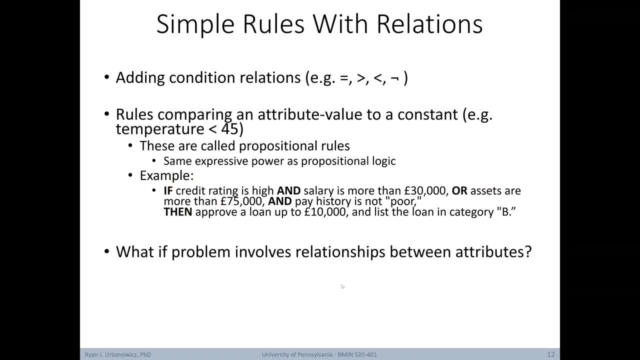 of this rule expression. But what happens when we want to look at a relationship between multiple attributes? These can't be expressed with simple propositional rules and a more expressive representation is required, similar to what we looked at as we went from propositional logic to first order logic. fortunately, we can do. 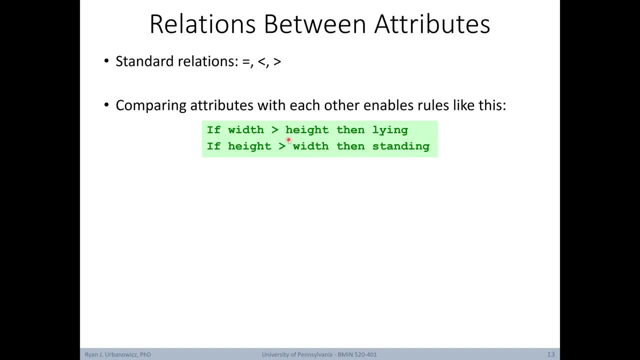 this pretty simply in rules. for example, if width is greater than height, then consequent is lying, or if height is greater than width, then consequent is standing. this is a simple example of rules that might be trying to determine how a person is positioned. this kind of rule representation. 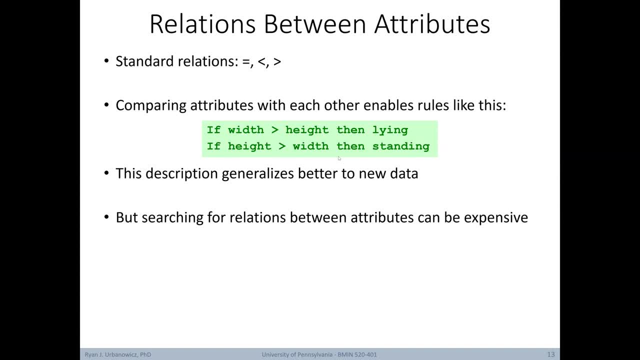 generalizes better to new data, but unfortunately, searching for relations between attributes can be computationally expensive. one simple solution is to add extra attributes via feature construction, for instance, to add an attribute that has already checked whether width is greater than height and have a true or false value. however, you can also use variables and multiple relations. 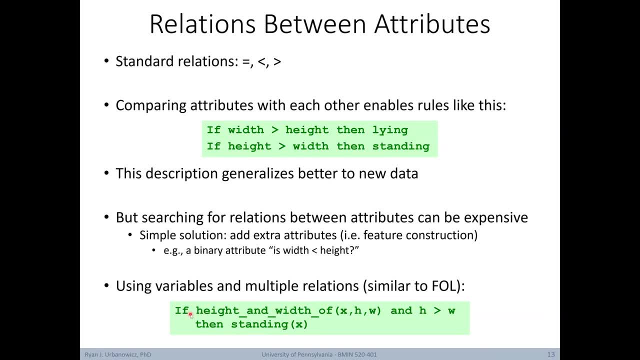 similar to what we saw on first order logic. for example, if height and width of xhw and asw are equal, then we can determine which is greater than xhw and which is greater than hw is greater than W, then standing Here, this expression indicates the height and 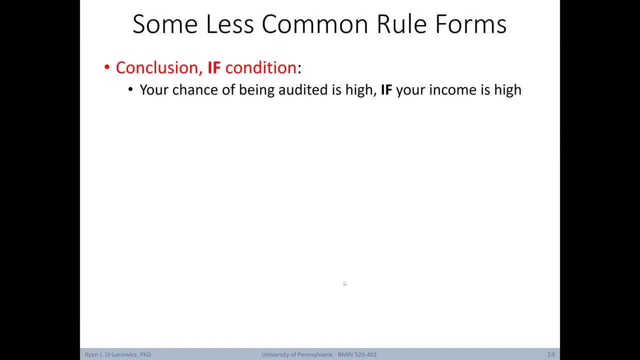 width of person X. It's worth noting at this point that there are also some other less common rule forms that you might encounter. For example, sometimes rules can be presented with the conclusion first given as conclusion if condition. So in other words, your chance of being audited is high if your income. 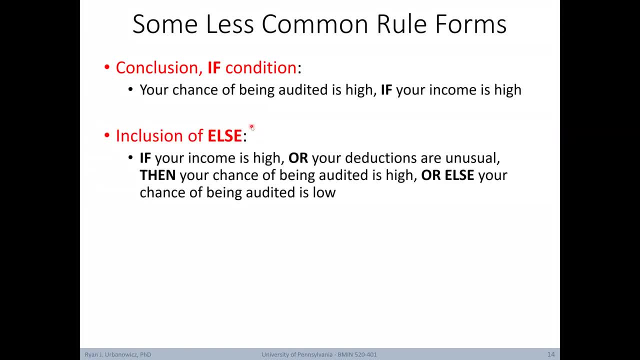 is high. You might also see rules that include the else expression. So, for example, if your income is high or your deductions are unusual, then your chance of being audited is high, or else your chance of being audited is low. This has 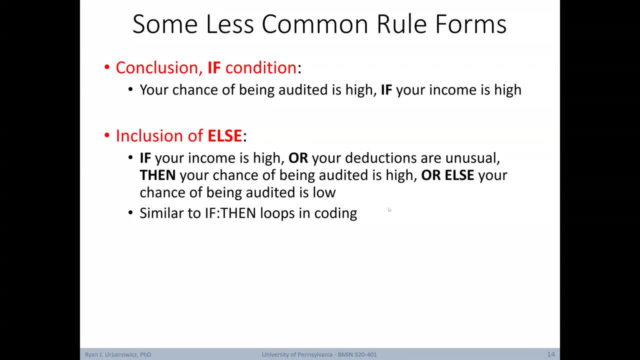 a similar structure to if-then-else loops that come from computer programming. You can also have situations where the action or consequent of a rule will actually trigger other rules or multiple actions. So, for example, you could have a rule that triggers, then approve the loan and refer to an agent. 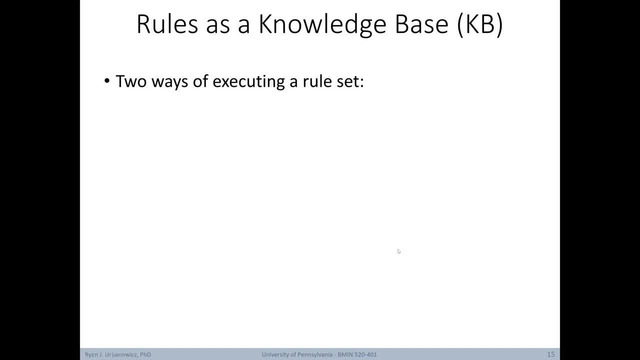 In this case, two actions are required. First, you have to think about the rules as a collective group that form a knowledge base from which we can work. First off, let's consider that there are two ways of executing a rule set. First, you can have an ordered set of. 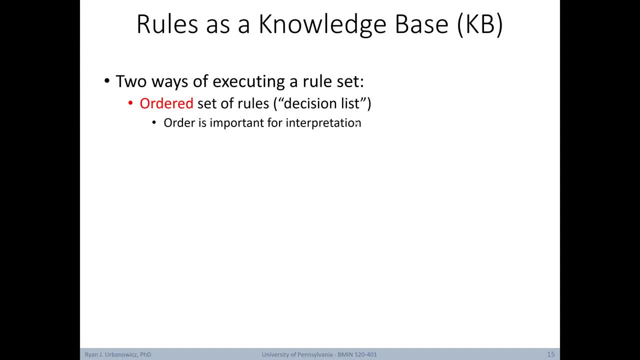 rules. This is also known as a decision list. In this situation, the order of rules is important, for how it's interpreted Differently. we can also have unordered rule sets. Here, rules can overlap and lead to different conclusions for the same instance. 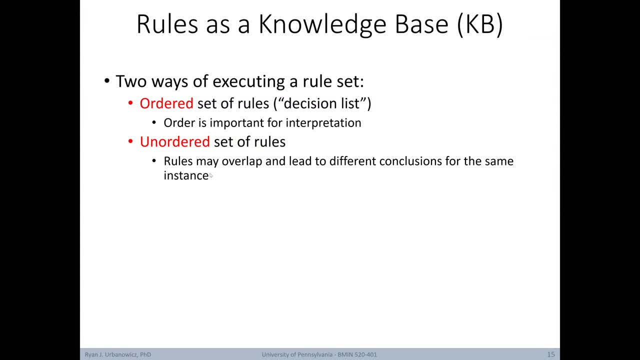 In other words, introduce conflicts. However, there are some benefits to having an unordered versus an ordered rule set. Another thing you can do with a knowledge base of rules is to rely on default rules. This tends to be common when using ordered rule sets. Basically, here, the idea is that you create rules. 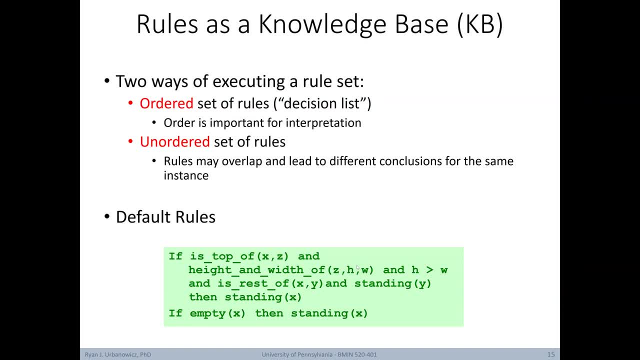 for other outcomes and if they're not satisfied, then a default rule with a default action or conclusion is triggered. Here's an example where a default rule is used. In this case, we have two rules, The second being a default rule that triggers whenever x is empty or no other. 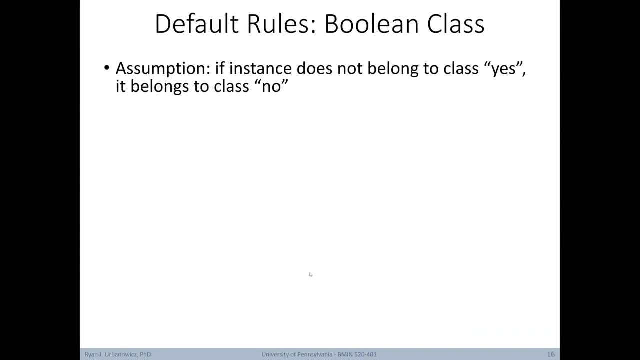 rules have triggered, giving us a consequent to work with. Let's look a little further at this idea of default rules from the context of problems where we have a Boolean class or Boolean outcome. So the assumption here is that if an instance doesn't belong to class yes, then by default it belongs to class. 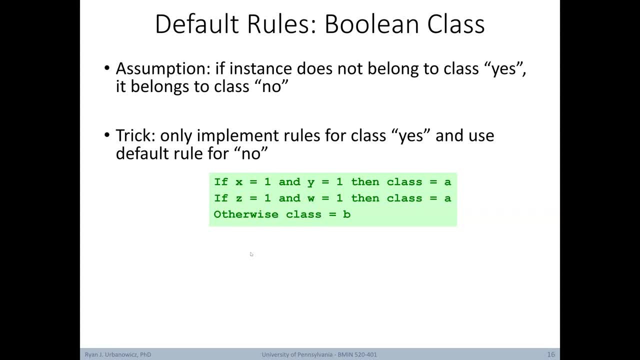 no. What's nice when we have this situation is that we only have to implement rules that indicate when we have a situation where class is yes and then just rely on the default. In this case, we only have to implement rules that indicate when we have a situation where class is yes and then just rely on the default. 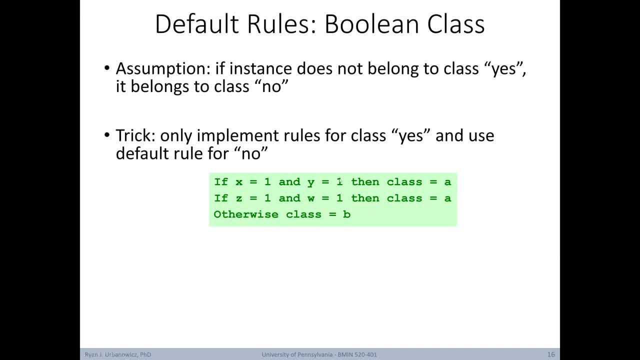 In this case, we only have to implement rules that indicate when we have a situation where class is no. In this example, our two classes of interest are class A and B, and so we've only provided rules that indicate when we're part of class A and otherwise the 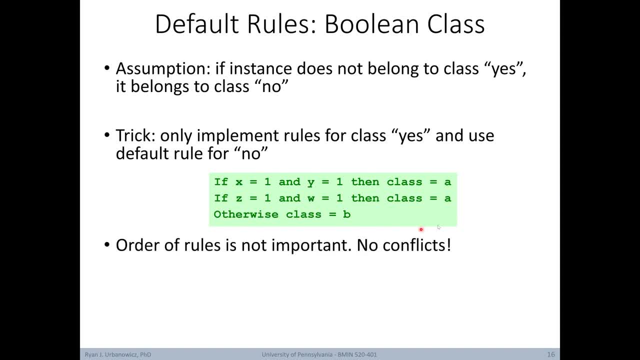 default rule of class B kicks on. In this situation, the order of the rules isn't important and we don't have any conflicts. Additionally, this set of rules is written as a disjunctive normal form. Specifically, we have two rules, both with. 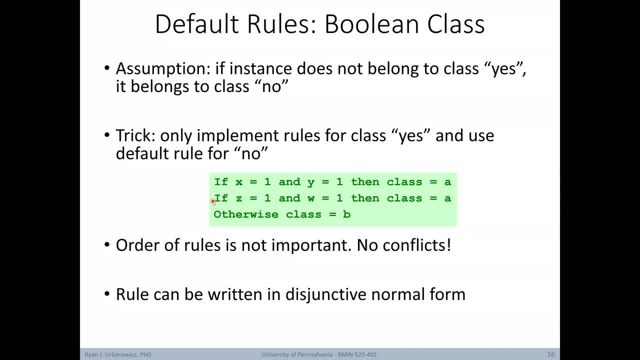 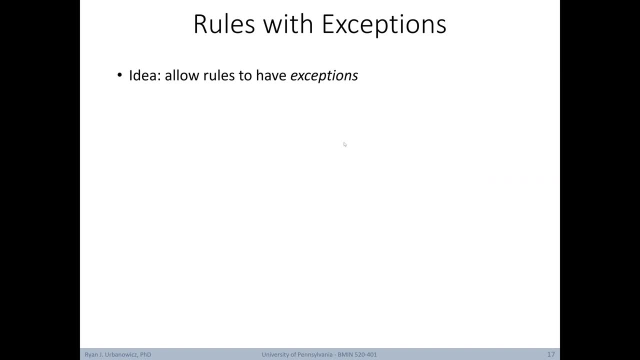 antecedents using and. but. either of these rules either or can be true in order to decide that we are of class A. Some uses of rules also allow exceptions. Let's take a look at an example: using the iris data set to get a. 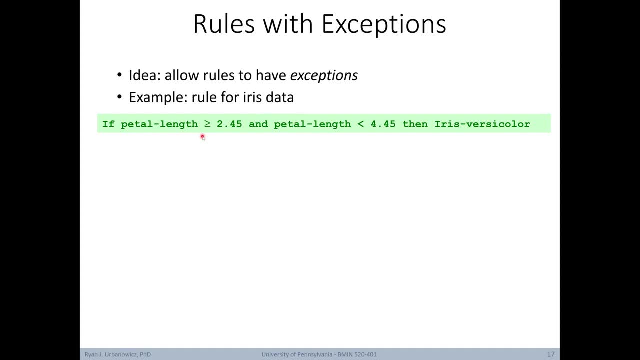 better idea of how we might use exceptions. So here we have. if petal length is greater than 2.45 and petal length is less than 4.45, then the iris class is iris versicolor. Let's assume at this point all the training. 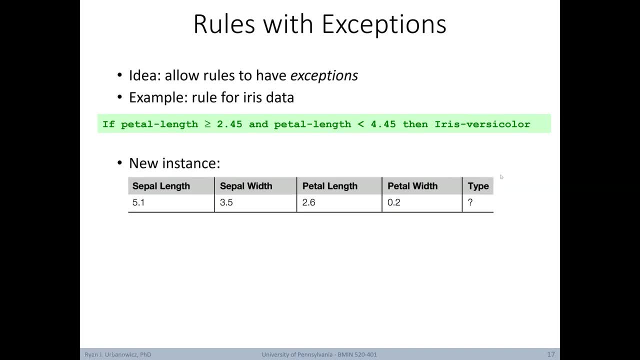 instances we've looked at backs this situation up. However, maybe another instance comes along that isn't part of class iris versicolor, Because the petal length here is 2.6, which would have fallen within this range. we could now come up with an exception to the above rule to make it. 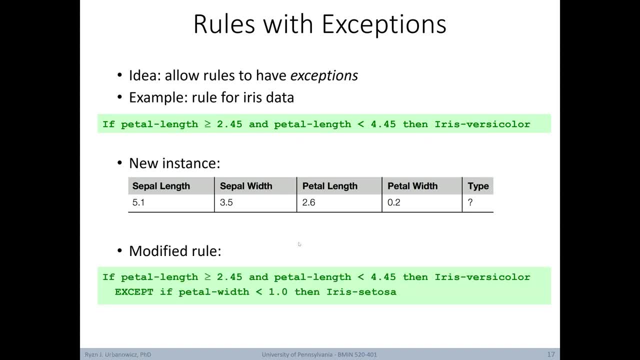 accurate in this new case. Here's the modified rule, with the exception. We've added the phrase except if petal width is less than 1.0, then classification is iris setosa. Here the presumption is that none of the other instances that were 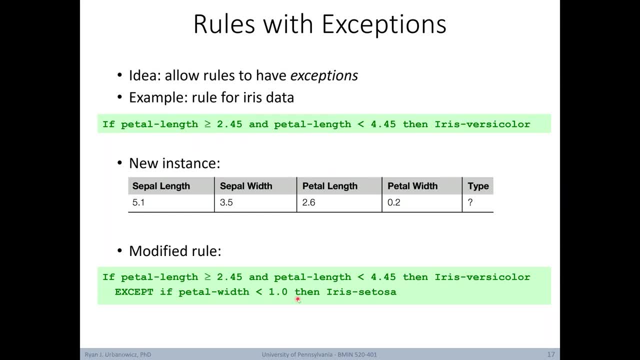 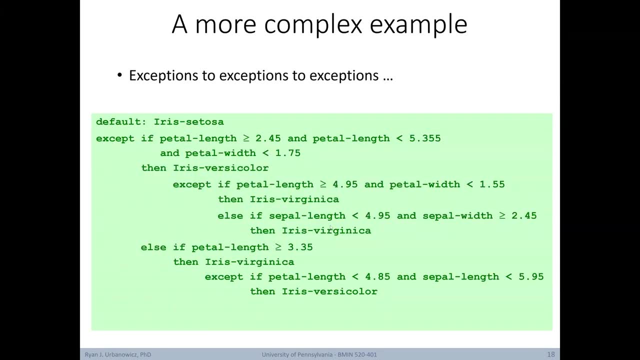 correctly classified here by this rule, meet the conditions of this exception. This can help us to deal with special cases in the context of rule-based systems. In practice, exceptions can get pretty unruly. Here's a more complicated example where a number of exceptions are used In this. 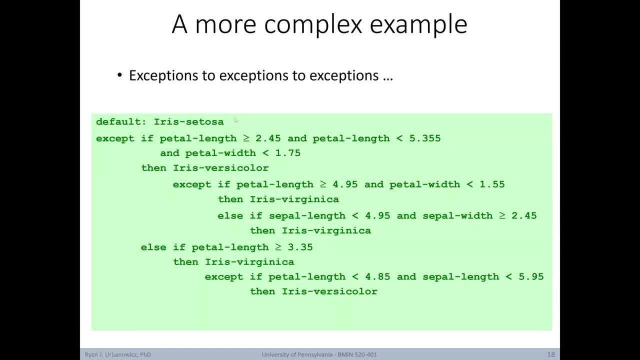 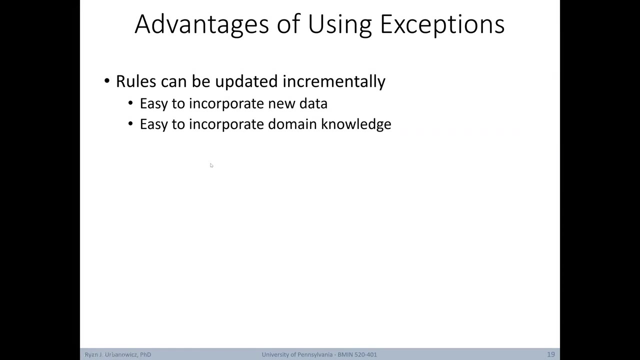 example, we're using the default rule kind of in reverse. We start with the default of iris setosa and then indicate exception conditions when we want to conclude a different class of iris, In this case iris versicolor and iris virginisa. The advantage of building rule systems using exceptions is that rules 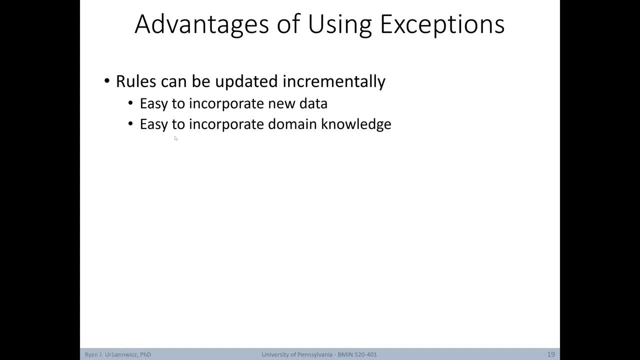 can be updated incrementally. In other words, it can be easy to incorporate new data or to incorporate new domain knowledge. In terms of interpretability, people often think in terms of exceptions. Further, each conclusion can be considered just in the context of the rules and exceptions that. 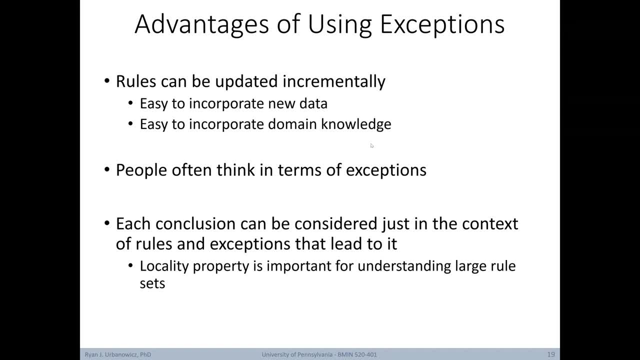 lead to it. This locality property can be important for understanding and interpreting larger rule sets. What we'll call normal rule sets don't offer the same level of transparency in terms of interpreting the rule base, So, while using exceptions and rules can be beneficial to interpretability, they can also lead to extreme overfitting when 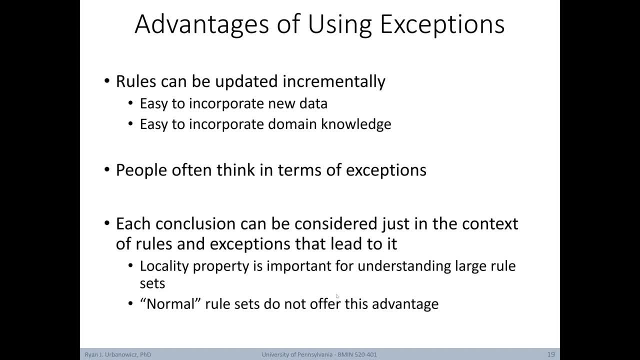 you're developing a rule set and they might require constant updates as new instances are introduced in the future. So, at the end of the day, this might not be the best approach in particularly noisy or complex problem spaces. Let's take a moment to look at the big picture of how a normal rule base might be set. 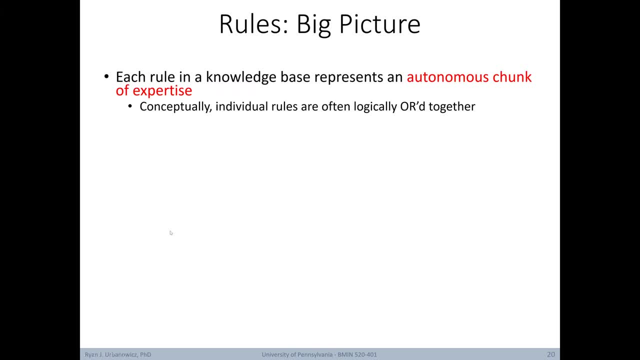 up and interpreted. Each rule in a knowledge base represents an autonomous chunk of expertise. Each individual rule is conceptually linked through or expressions. When these rules are combined and fed into what's called an inference engine, the set of rules behaves synergistically, being utilized collectively to make decisions and 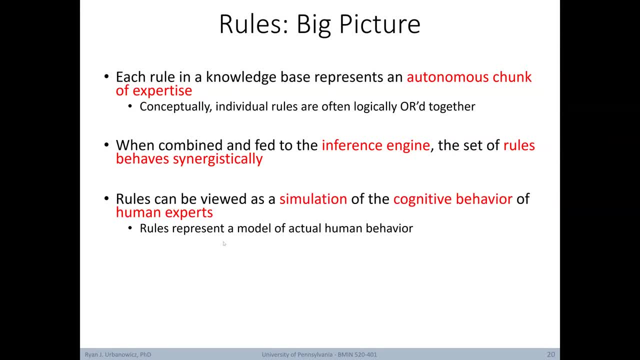 choose new actions. The use of rules can be viewed as a simulation of the cognitive behavior of human experts Or otherwise put, rules represent a model of actual human behavior. As such, they're a predominantly used technique that's used to formulate knowledge in expert systems And, furthermore, they're often used in 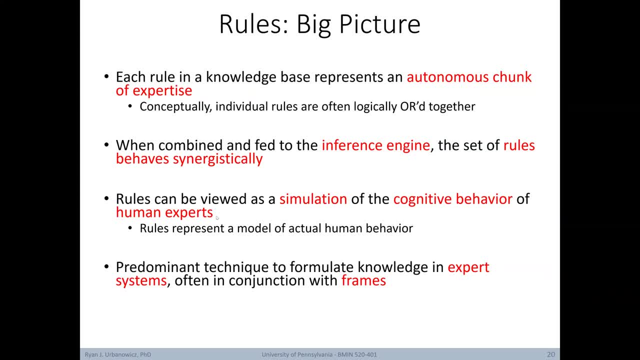 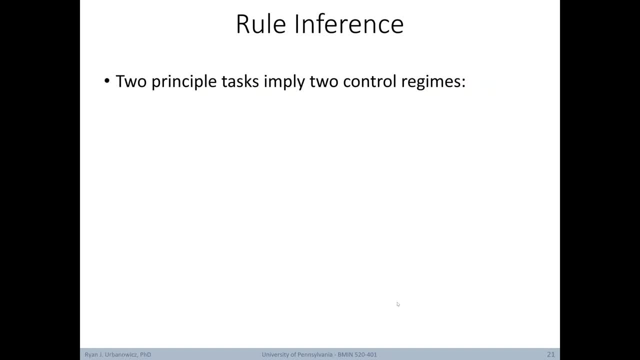 conjunction with frames in the construction of expert systems. We'll get a taste of expert systems at the end of this lecture, but we'll dive into them much further in our next lecture. Now that we know the basics of what rules are and how they can be represented, let's take another big-picture look at. 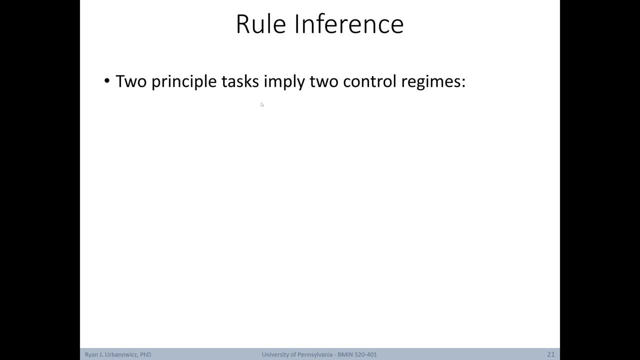 how they can be applied to make inferences In terms of the problems we might be trying to address. there are, in general, two principal types of tasks that imply the use of one of either two control regimes. The first control regime is forward chaining. This is a data-driven approach that we learned a. 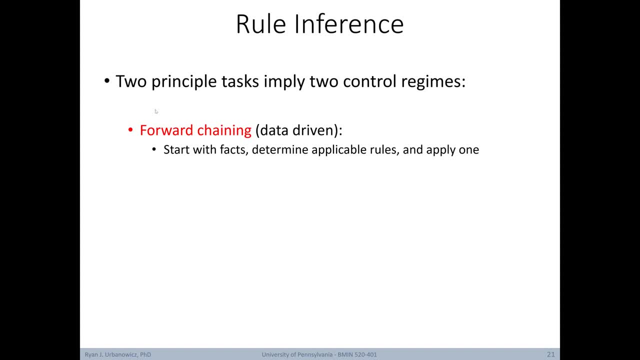 little bit about in logic. Here we start with facts and determine applicable rules and then apply one. There's also backwards chaining, which we learned a little bit about in logic, which is goal-oriented. Here we look for rules which decompose the goal And then we try to solve secondary, subsequent goals. 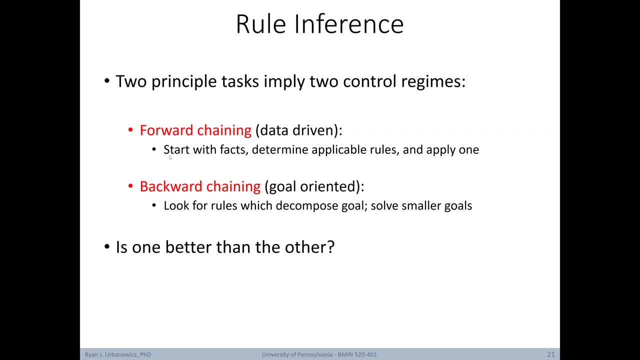 until we've proven our original goal. You might initially wonder whether one of these control regimes is better than the other, but the answer to that question really depends on the application and the circumstances. As such, both are useful approaches that we'll want to keep in. 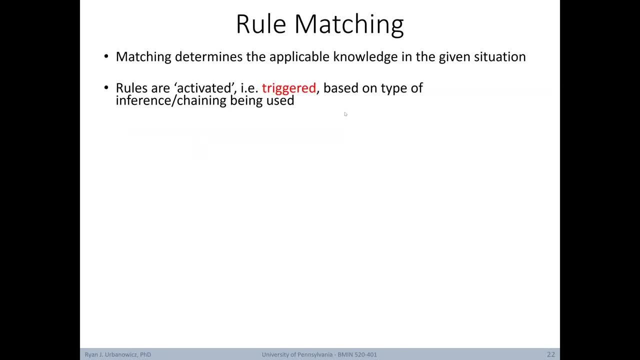 mind. An important part of using rules to make inferences is the process of rule matching. Matching is all about determining the applicable knowledge of the given situation. In other words, based on the knowledge at hand, which rules are relevant to look at. further, Rules become activated or triggered. 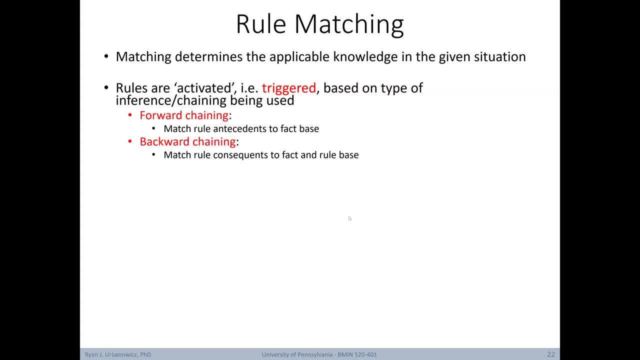 based on the type of inference or chaining being used. In forward chaining we're trying to match rule antecedents to the fact base that we have in hand, whilst in backwards chaining we're trying to match rule consequence to facts and the rule base to see if we can either prove that our consequent is true. 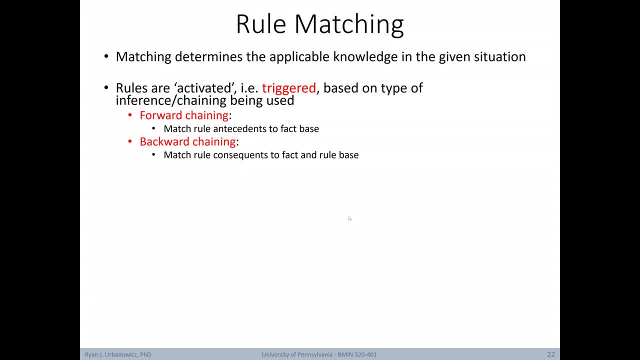 or find other rules that match that consequent, so we can use those other rules to try and prove its truthfulness. However, it's this process of matching that can be the most computationally expensive. Further matching often yields more than one applicable rule. that needs to be. 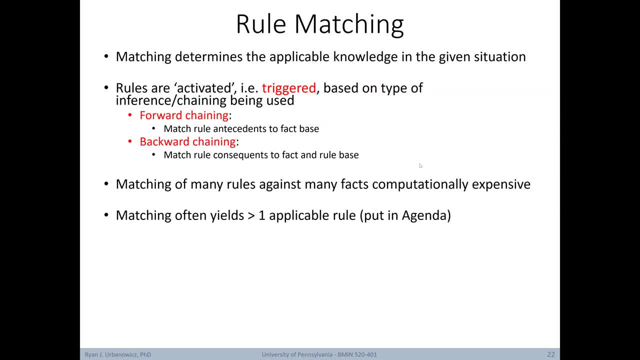 considered and in those cases it would be put on an agenda of rules to be looked at in sequence. When multiple rules are applicable, these rule instances are said to be in conflict and we need to use conflict resolution to pick one to fire. 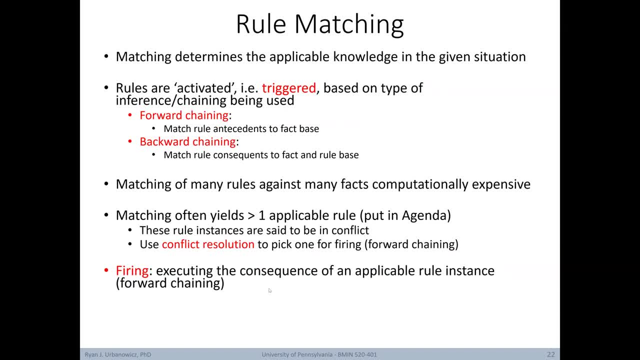 Firing is a term used in forward chaining to describe the execution of consequence of an applicable rule instance. In other words, if the antecedents of a rule are satisfied, then the consequent is added as a new fact through firing. It's also during the matching process that variables and rules 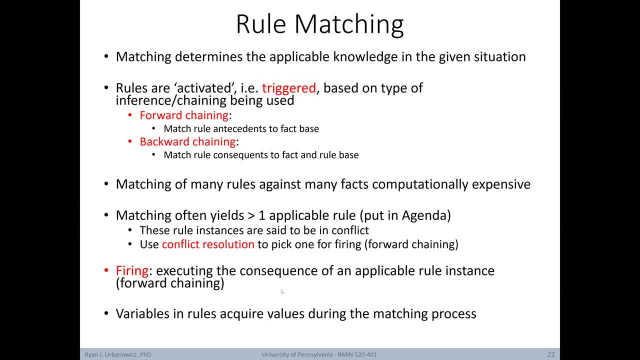 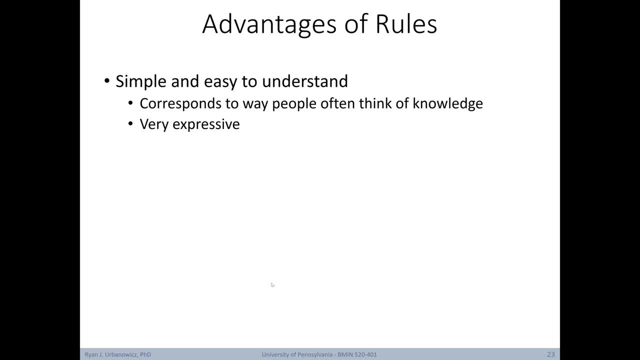 acquire values like instantiation from logic. So what are the advantages of rules as a representation on a whole? Well, first, they're simple and easy to understand and naturally correspond to the way people often think of knowledge. Furthermore, they're very expressive. Another advantage is that rules are 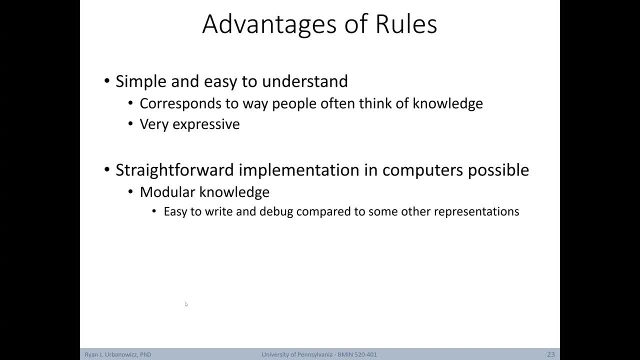 straightforward to implement in computers and they allow for the modularization of knowledge, So an engineer of the system can just focus on the validity of individual rules, one at a time, more than having to worry about a giant conglomeration of if-then-else loops or some other more complex type of model. 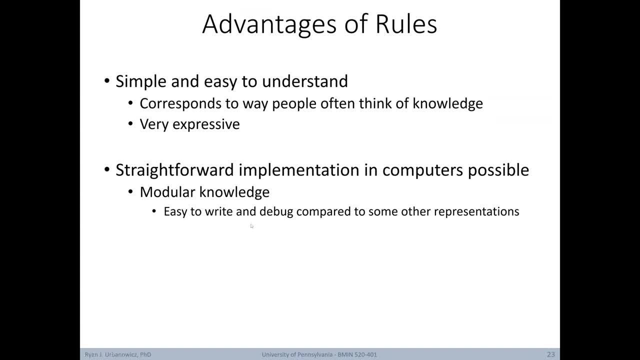 So ultimately, rule-based systems are also easier to write and debug compared to some other representations. Another nice thing is that there are some formal foundations with respect to inference, for example, for some of the variants of rule-based systems, but not all of them. The more creative you get. 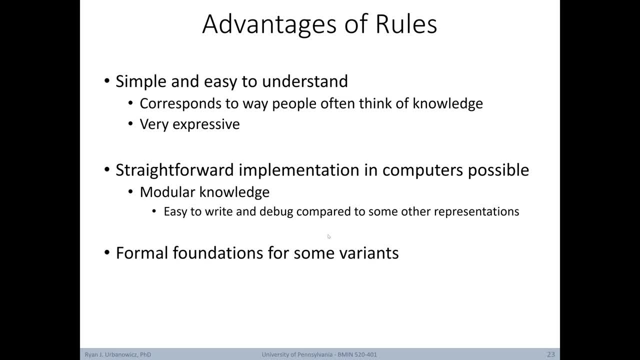 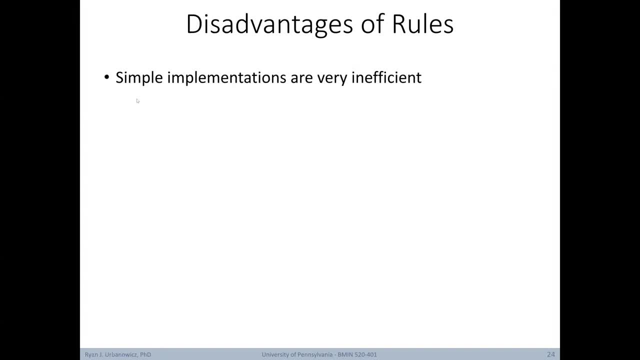 in putting together a rule-based, the farther you stray from a formal system that allows you to make reliable inferences. Now let's review some of the disadvantages of rules. as a representation For one, simple implementations of rules are often very inefficient. In other words, we can modularize our problem too much to make our lives easier. in putting 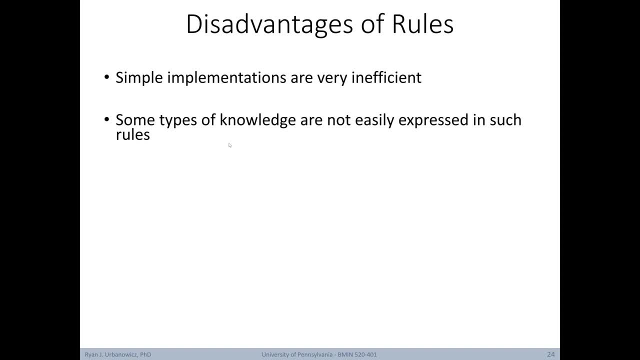 together the system, but when it comes to putting it into action, that same system might be computationally more expensive than it needs to be to go through the whole searching, matching and inference process. Also, some types of knowledge are not easily expressed as rules. 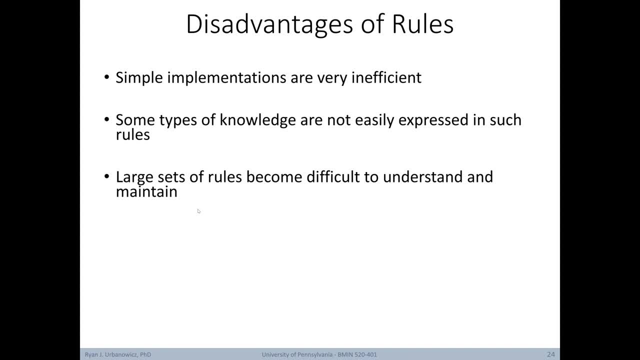 Further, a large set of rules can become difficult to understand as well as to maintain. Rule-based systems can also be memory-intensive as well as computationally expensive, And, at the end of the day, they can still be difficult to debug, since we might have 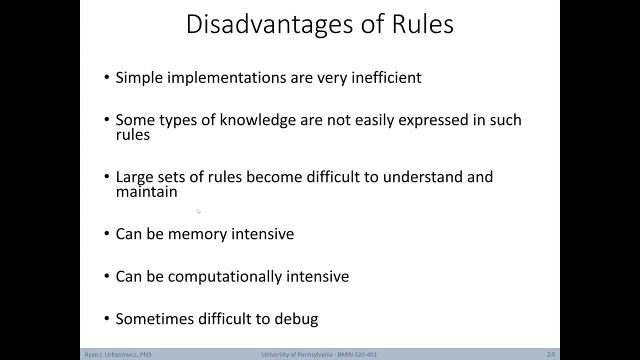 to consider the nuances of how rules work together, ultimately to make inferences, rather than just being able to focus on the validity of individual rules, one at a time. Subtitles by the Amaraorg community. In other words, when rules start to have important interactions between them, that 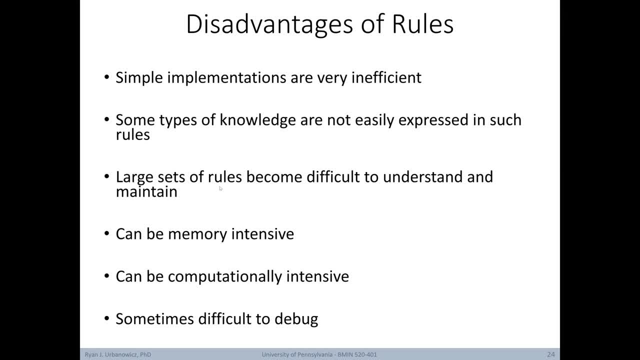 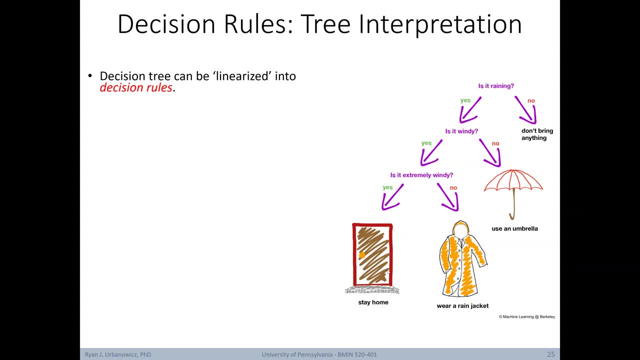 can influence the validity of the implications that we're making through the system as a whole. Now that we've learned about rules, let's go back to our discussion of decision trees and tie the two together. First off, any decision tree can be linearized into what are called decision rules. 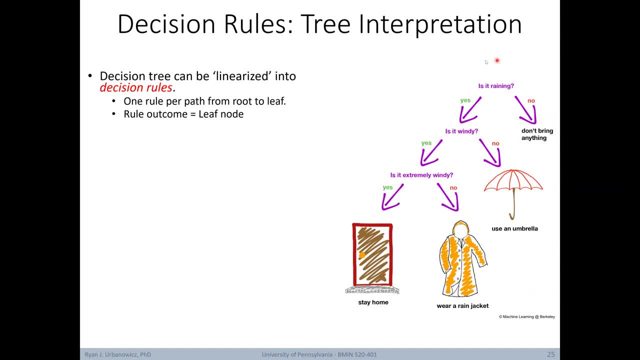 You can create a decision rule from every unique path, from the root of the tree to a given leaf. So, for example: is it raining? Yes. Is it windy? Yes. Is it extremely windy? Yes, Stay at home Here. the leaf node would be the outcome of that rule describing this entire path up. 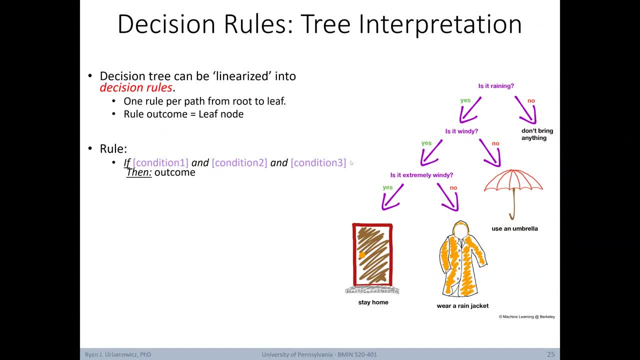 through the tree. As we've seen, rules are if-then expressions. Here are some examples of decision rules we would get by linearizing this example tree. So, for instance, if not raining, then don't bring anything, would represent this part of. 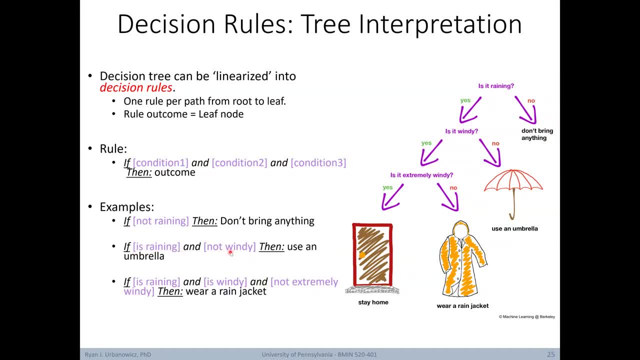 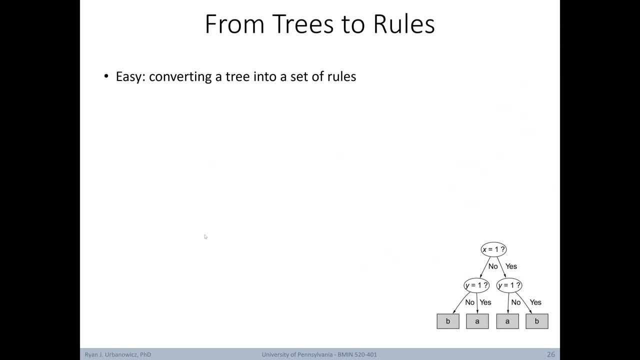 the tree. If is raining and not windy, then use an umbrella would represent this part of the tree. If is raining and is windy, and not extremely windy, then wear a rain jacket would represent this part of the tree. Converting from trees to rules is extremely easy. 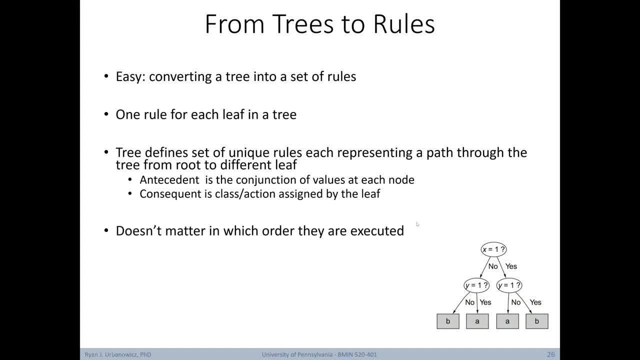 Again, you just get one rule for each leaf in the tree. One nice thing about the rules that you get from a tree is that it won't matter what order they're executed in. However, the resulting rule set that you get from decomposing a tree could be unnecessarily. 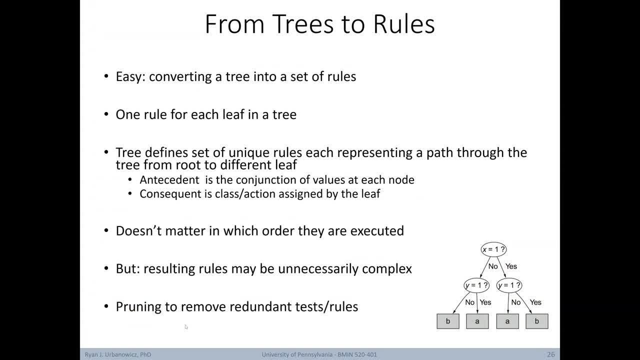 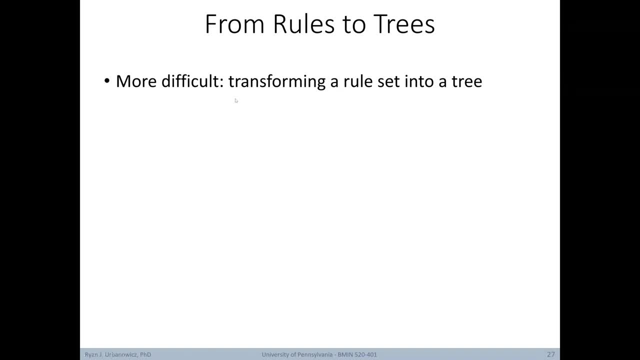 complex. In order to avoid this, you could prune a tree or a rule set to remove the leaves from the tree, Or you could prune a tree or a rule set to remove redundant tests or rules. What about going from rules to trees? This is actually much more difficult. 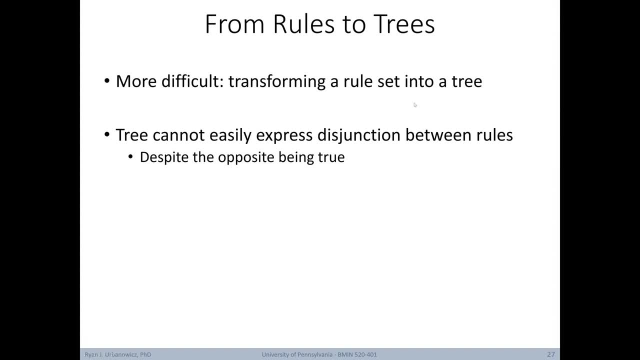 A tree cannot easily express a disjunction between rules, despite the opposite being true. Further, a given rule base might not have the same sub or superset of attributes required to assemble a representative tree structure. So, for example, keep in mind that when going from trees to rules, all rules will have the 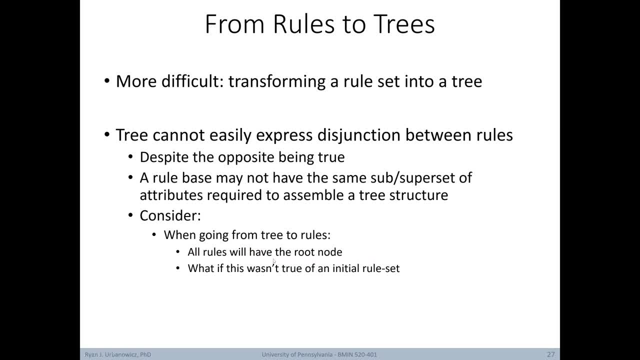 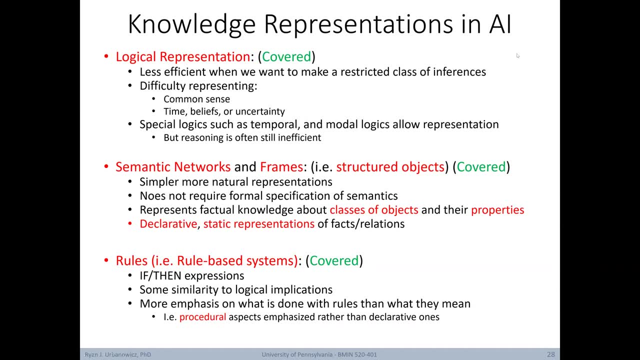 root node. The root node must be specified as part of its antecedent. So what would we do if this wasn't the case? in our initial rule set that we wanted to turn into a tree. At this point we've covered all of the major forms of knowledge, representation and 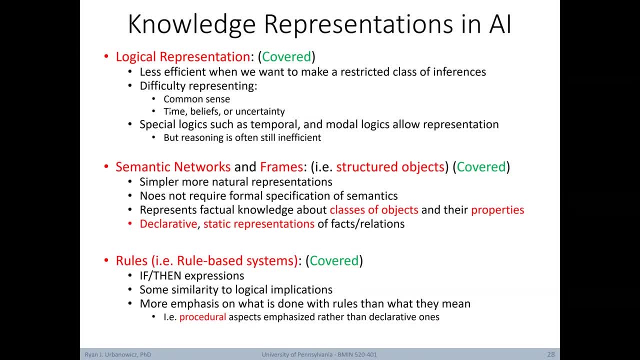 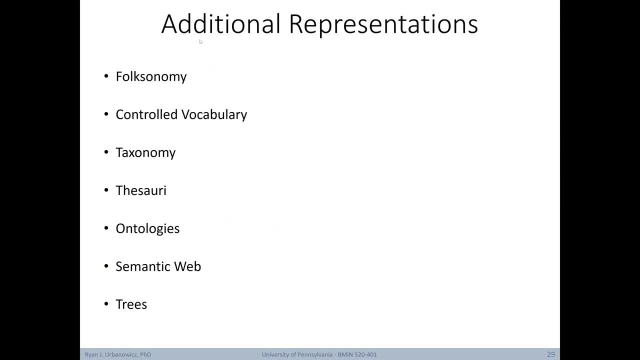 AI that are used today. However, this is not an entirely exhaustive list, Just a list of the ones that are used most frequently, And here's just a reminder of some of the many knowledge representations we've considered in general so far in this course. 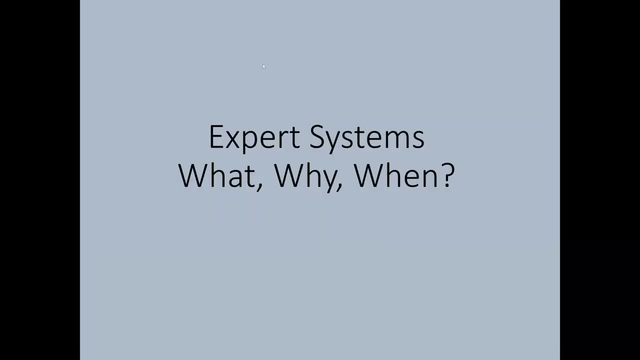 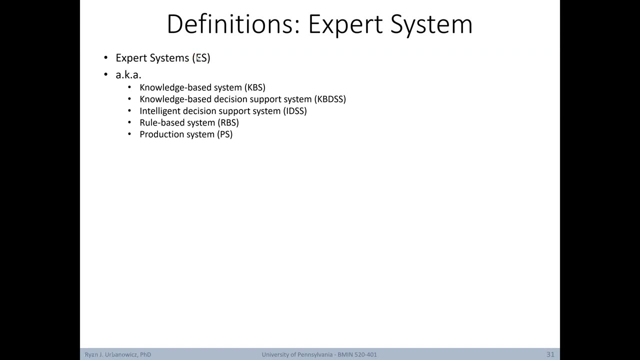 All right, so now we're going to shift gears and start talking about expert skills. Let's talk about expert systems, beginning with the what, why and when. The term expert system can be abbreviated by ES, and it can go by a number of names. 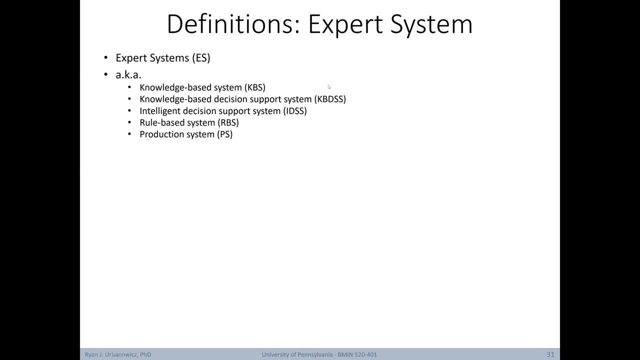 A knowledge-based system, a knowledge-based decision support system, an intelligent decision support system, a rule-based system or a production system. Now, these names aren't entirely equivalent, but when you hear them, the first thing you should think of is expert system. 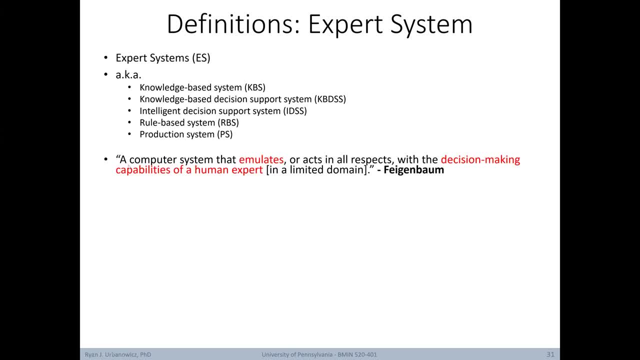 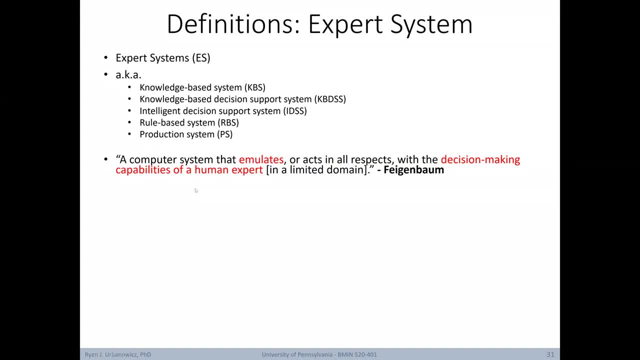 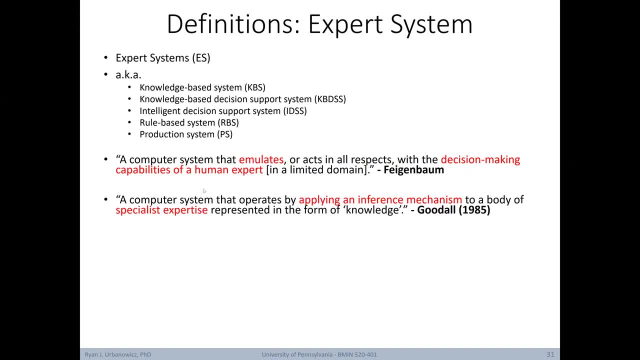 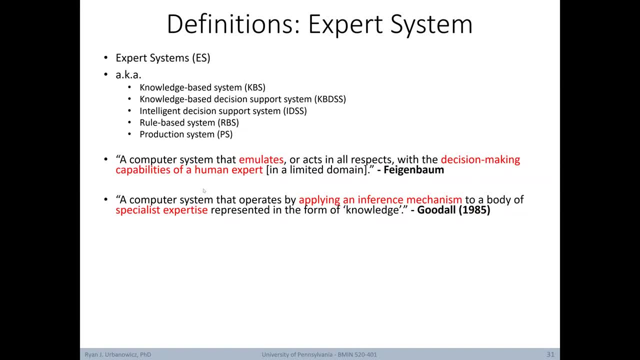 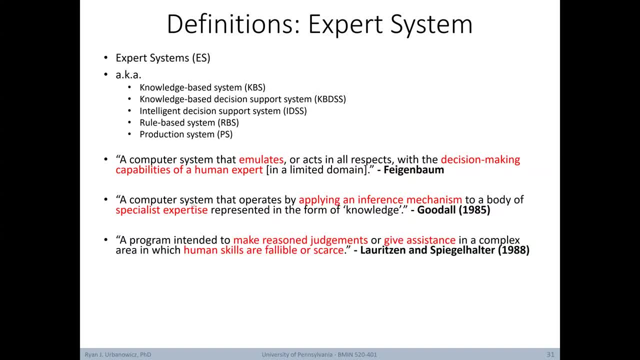 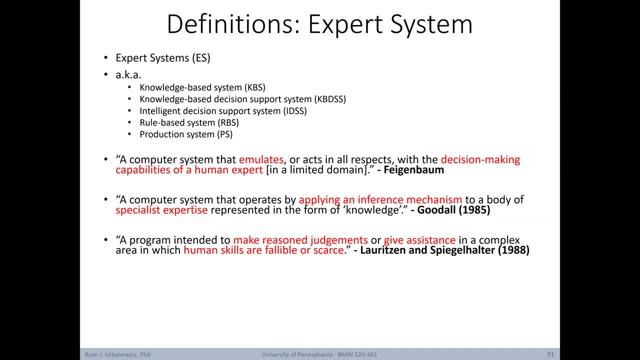 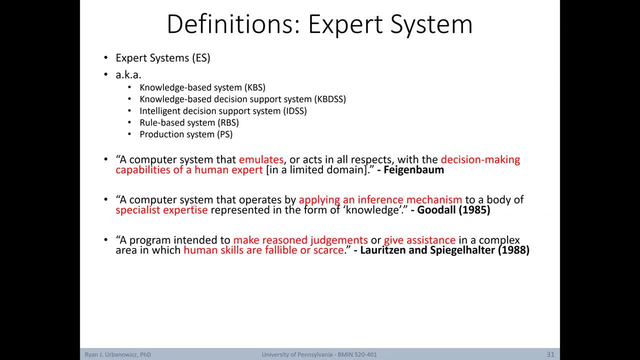 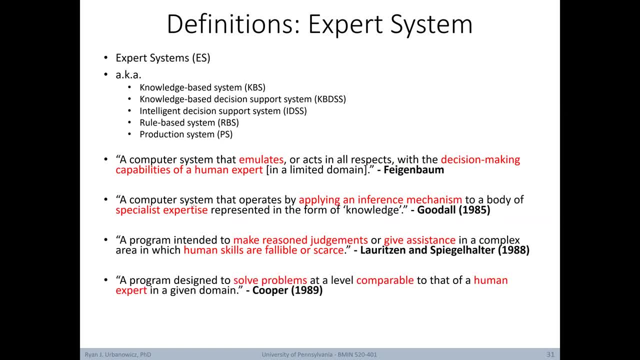 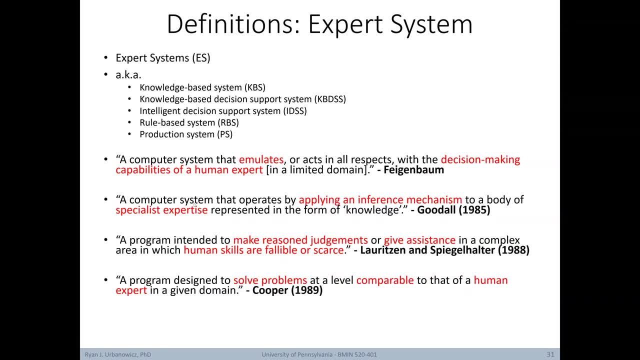 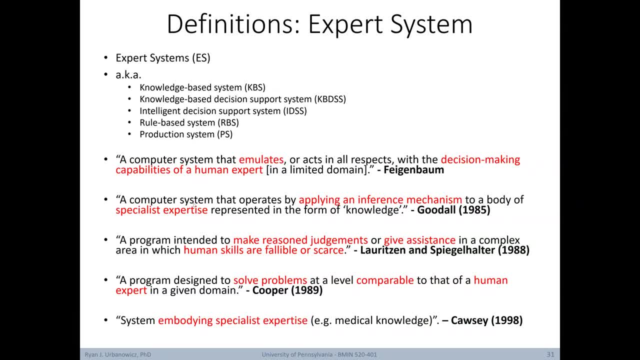 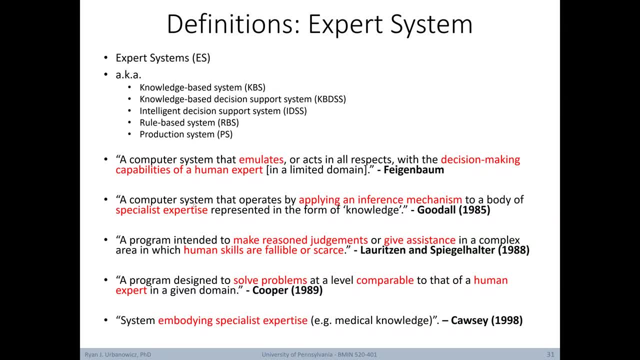 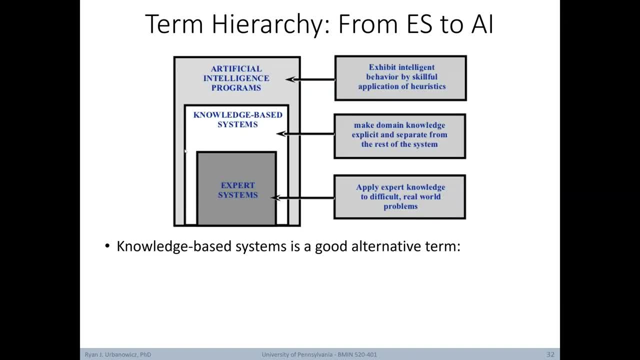 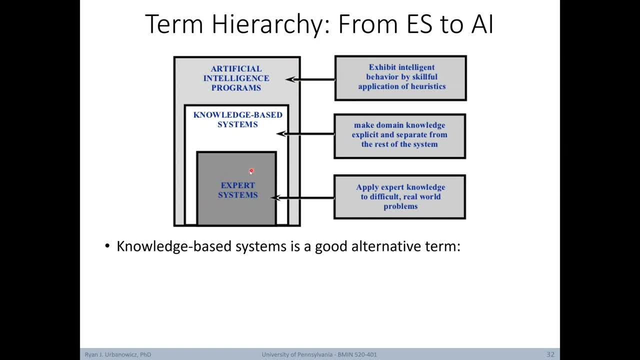 of artificial intelligence programs. You might hear the terms expert systems and knowledge-based systems used largely interchangeably. However, the distinction is that expert systems tend to focus on knowledge that is considered expert level, The thing that distinguishes knowledge-based systems from artificial intelligence programs. 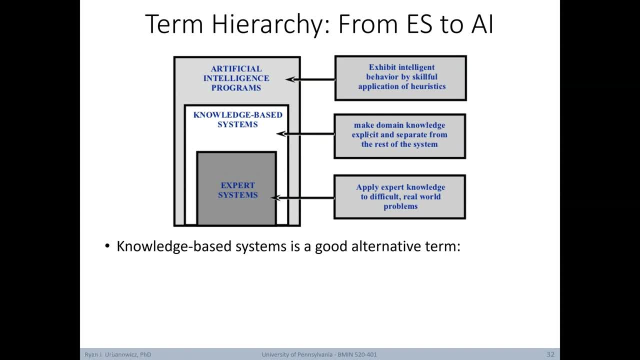 is that knowledge-based systems make domain knowledge an explicit separate resource from the rest of the artificial intelligence system. So, in particular, expert systems store all of their knowledge and relations in a separate knowledge base And then the reasoning component stands alone as its own separate entity that can work on that knowledge base. 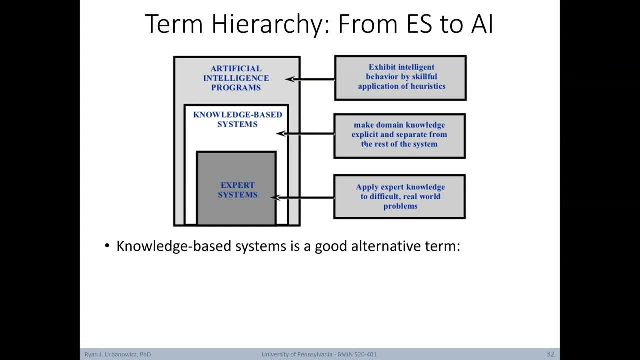 This aspect is what distinguishes a knowledge based system from the rest of artificial intelligence work. In this course, we'll tend to use the term expert system, but you can basically think of them as being synonymous with knowledge based systems for the purposes of this course. 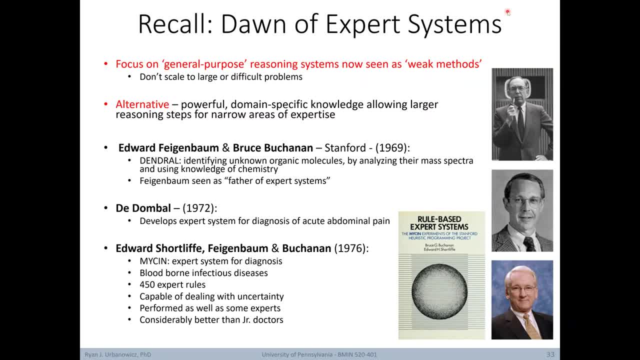 Recall from our lecture on the history of artificial intelligence, we had this slide describing the dawn of expert systems. We saw the birth of such systems begin in the late 60s and accelerate through the 70s. The earliest systems had a distinct focus on scientific problems, including organic chemistry and diagnosis in the medical fields. 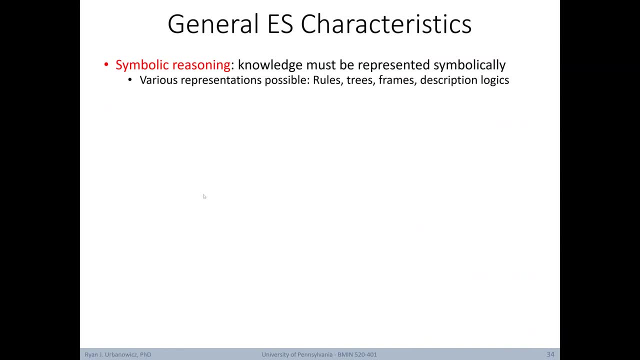 At a really high level. what are some general characteristics of expert systems? Well, first and foremost, they utilize symbolic reasoning. In other words, knowledge must be represented symbolically through things like trees, rules, frames or description logics. Expert systems also apply heuristics to guide the reasoning in an attempt to reduce the search area for a solution. 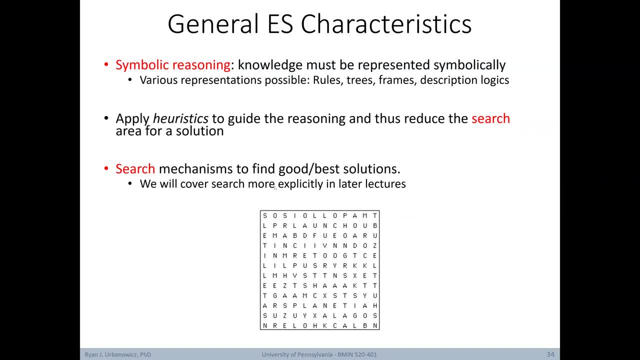 Search is an essential aspect underlying how these systems operate, with the goal being to find good or the best solutions. We'll be covering search in depth in a later module of this course. Now let's think about you. What are expert system characteristics, in contrast with other artificial intelligence systems? 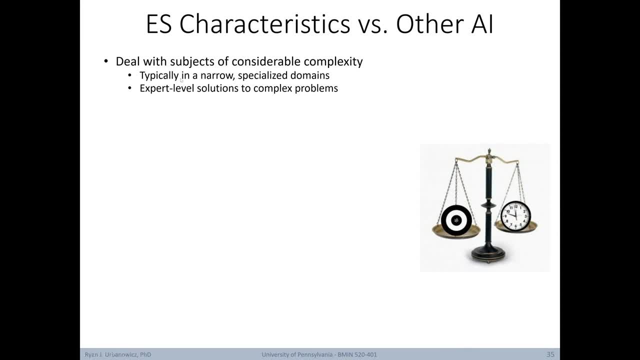 First, expert systems tend to deal with subjects of considerable complexity. Typically they're focused in a narrow specialized domain and they provide expert-level solutions to complex problems. So, at the end of the day, expert systems aren't typically focused on automation or convenience of trivial tasks. 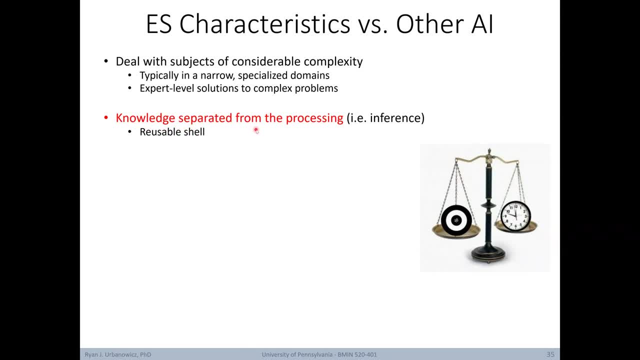 As I implied before, the knowledge in expert systems is separated from its processing, or in other words, the inference. This gives us a reusable shell framework for these systems that can make it easier to plug and play an expert system framework and adapt it to solve entirely new problems. 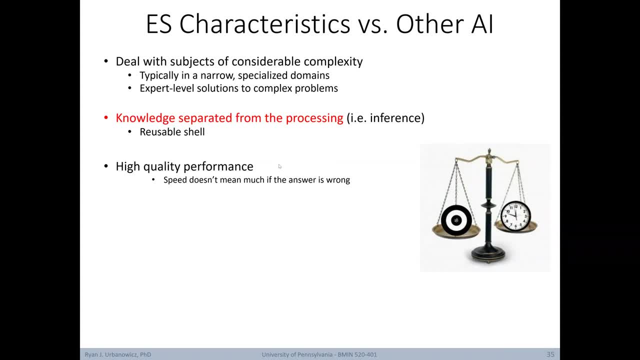 Another thing that's emphasized in expert systems is the need to have high-quality performance. The mantra here is that speed doesn't really mean that much if you get a wrong answer. However, with that in mind, it's still important that our expert systems be as fast as possible. 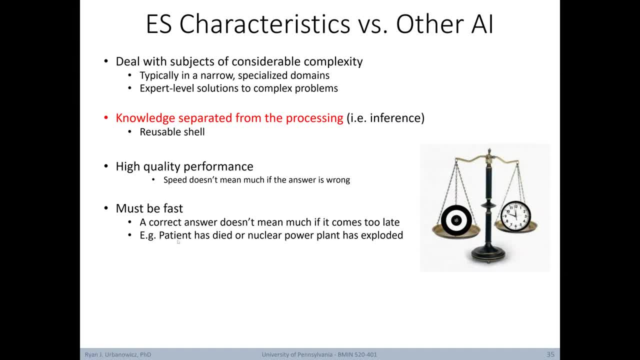 Because a correct answer doesn't mean much if it comes too late, For example, if a patient has already died or a nuclear power plant being controlled by an expert system has exploded. Another commonly important aspect of expert systems is that we want them to be capable of explaining and justifying the solutions they come up with. 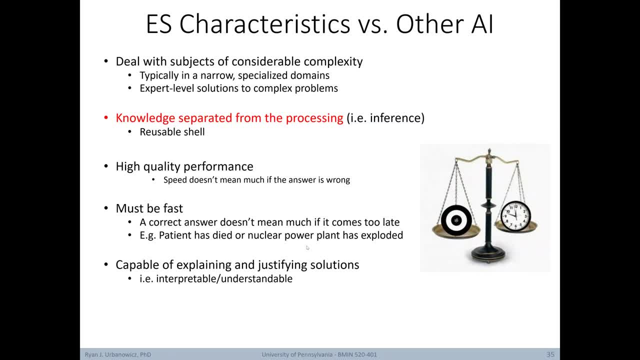 This is just another way of saying that we care about their interpretability or their understandability. And, lastly, we want them to be flexible. Often, expert systems are focused on domains where new information might need to be incorporated. where new information might need to be incorporated. 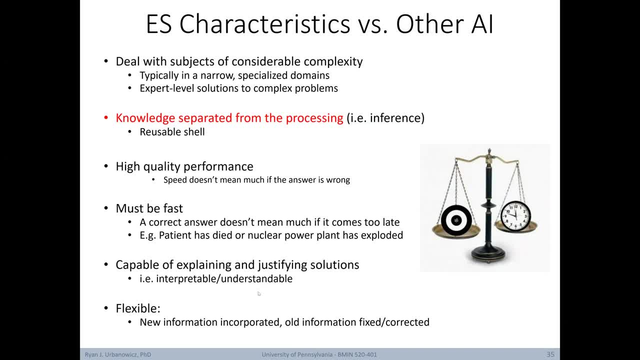 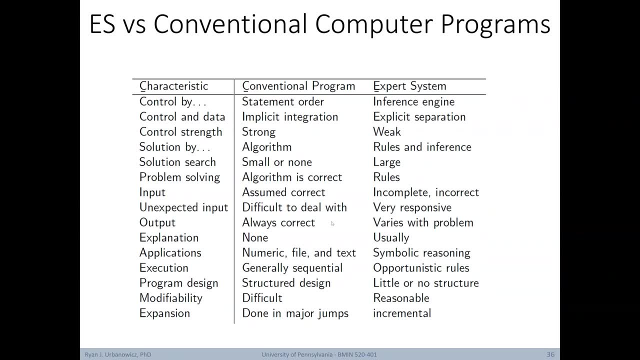 where new information might need to be incorporated or old information might need to be fixed, corrected or updated. Here's a table that tries to outline some of the major differences between thinking about an expert system versus thinking in traditional computer programs. For example, when it comes to control and data, conventional programming implicitly integrates the two. 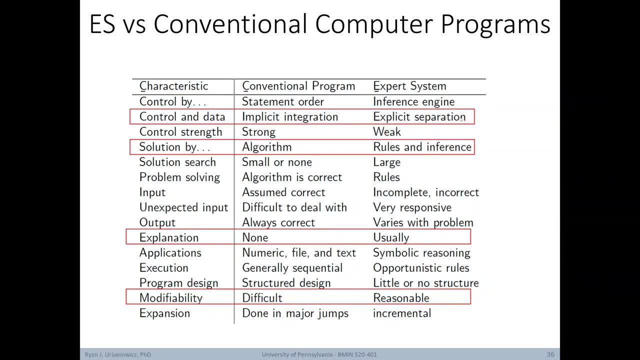 while expert systems explicitly separate them, as you've just heard. In conventional programming, a solution is usually reached using an algorithm, while in an expert system, it starts from inference on rules. Also, when it comes to explanation, conventional programs usually don't have a mechanism to do this. 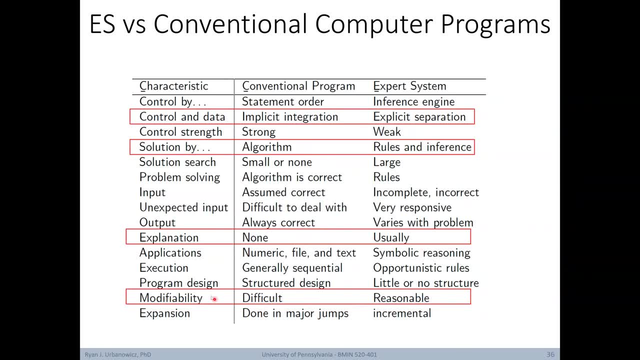 but in expert systems this is usually an important aspect. And lastly, looking at modifiability, conventional programs are usually difficult to modify, while expert systems usually offer a more reasonable, easier path. Here is a high-level schematic of an expert system. 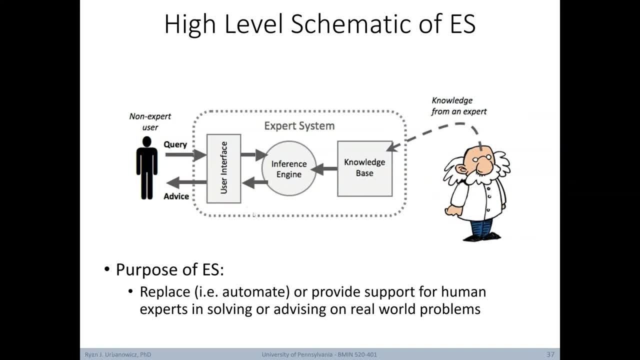 While everything inside this dotted line is part of the expert system itself, we have a non-expert user who can query the system and get advice back, and we have a knowledge base in the expert system that has been assembled based on the knowledge from expert human beings in the real world. 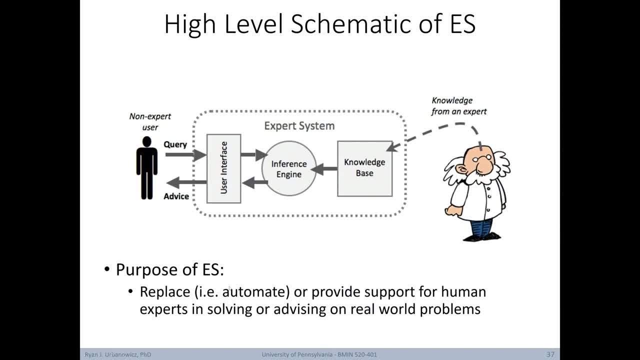 Ultimately, the purpose of an expert system is to replace, in other words, automate or provide support for human experts in solving or advising on real-world problems. There are two main components of an expert system, the first being the knowledge base itself. 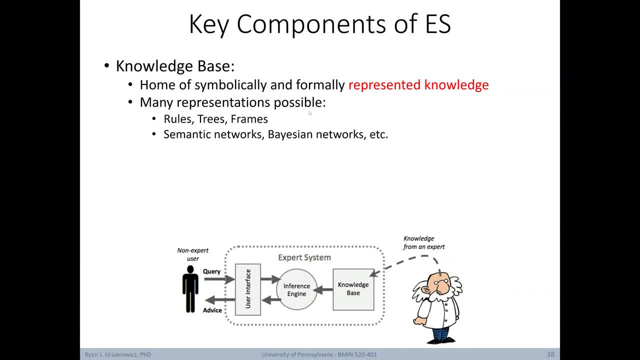 This is the home of symbolically and formally represented knowledge that can take on many representations, as we've mentioned, The second key component is the inference engine. This is responsible for reasoning, in other words drawing conclusions from the knowledge base Critically. the reasoning or inference approach must pair with the representation being used. 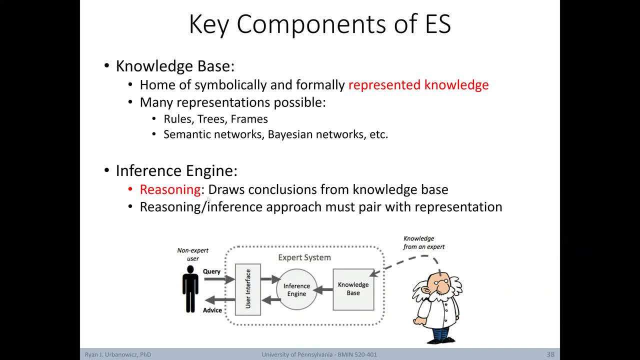 So if you have an expert system that was designed to work with rules, you couldn't simply replace them with trees or frames without expecting some major issues that might need to be resolved or thinking about completely redesigning the expert system from scratch, In addition to those key components. 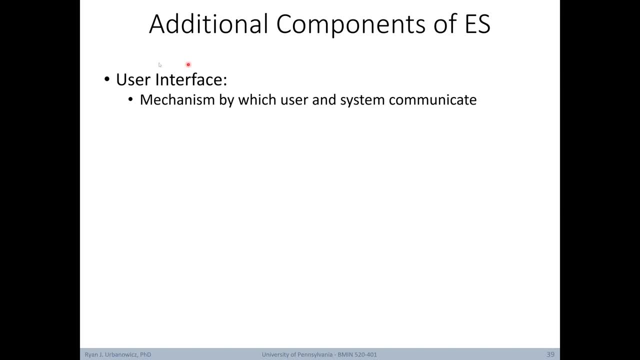 there are also some other common components of an expert system. For one, a user interface. This is just a mechanism by which the user and the system can communicate with one another. Another common component of an expert system piece of software is a knowledge base editor. 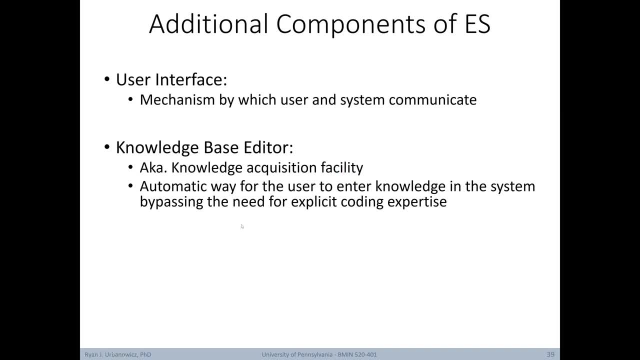 This is also known as a knowledge acquisition facility. This basically provides an automatic way for the user to enter knowledge into the system, bypassing the need for explicit coding expertise. Basically, at the end of the day, it's easier for non-computer science experts to help maintain, improve and update an expert system. 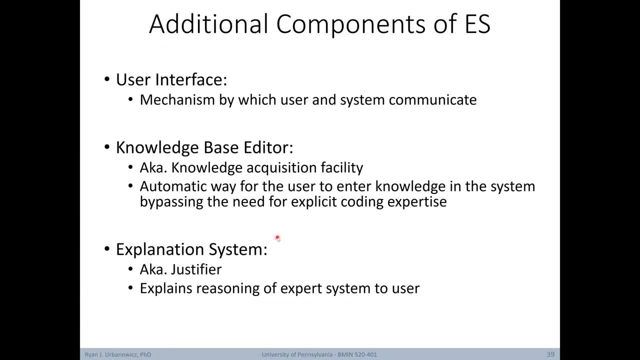 And lastly, expert systems often have a component of an explanation system. This is also known as a justifier. This component is responsible for explaining the reasoning of an expert system to a user in the form of some natural language or something as close to natural language as possible. 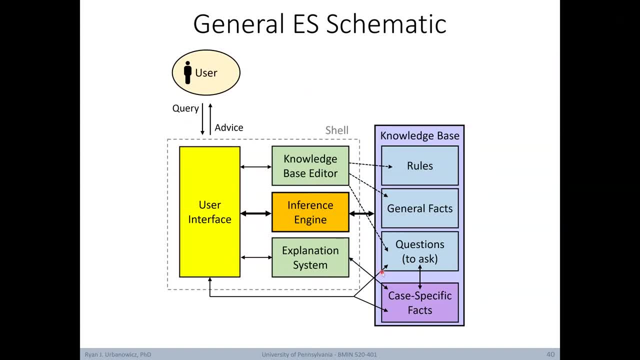 Here's a schematic I've put together to try and better capture all of the different aspects of a typical expert system. Again, on the outside we have a user who can ask queries and get back advice and they're interacting with some user interface. 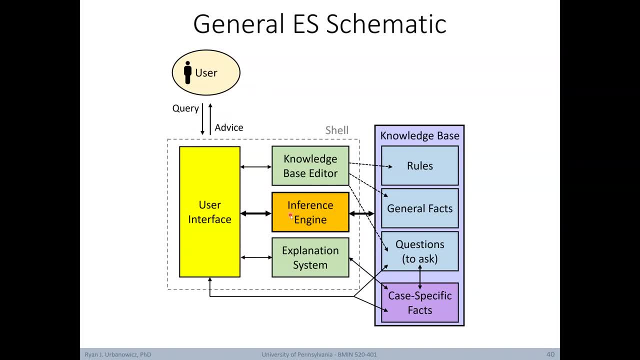 This user interface is importantly connected to the inference engine, as well as possibly being connected to a knowledge base editor and an explanation system, if they're available. in that expert system implementation. Notably, all of these items belong to a shell. This is a reusable part of an expert system. 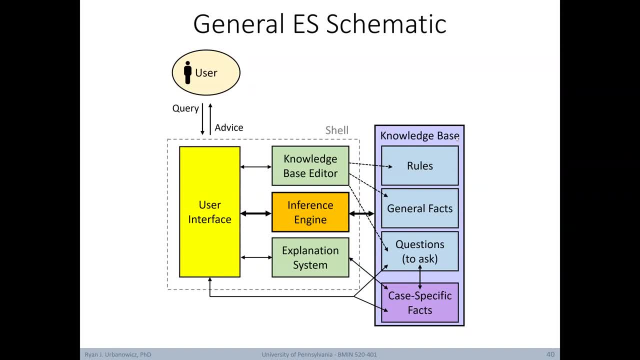 From here, the inference engine is connected to the knowledge base. This is made up of rules, general facts, questions that might be needed to ask the user and a temporary memory space for case-specific facts or new facts that can be added when investigating a specific query from the user. 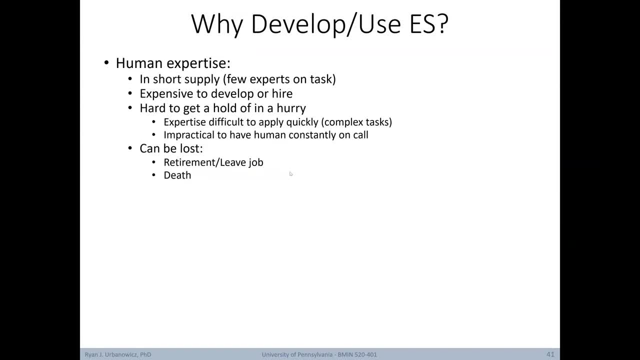 Putting together an expert system isn't a trivial affair, So why do people take the time to develop or use them? Well, first off, when it comes to human expertise, it's often in short supply. There might be only a few experts in the world to begin with. 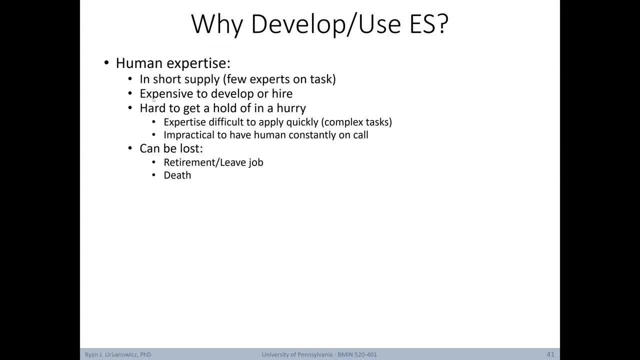 or only a few available to work on the task. Such experts can be expensive to develop or to hire, or they could be simply hard to get a hold of in a hurry. Sometimes even an expert has trouble applying their knowledge quickly, especially in very complex tasks. 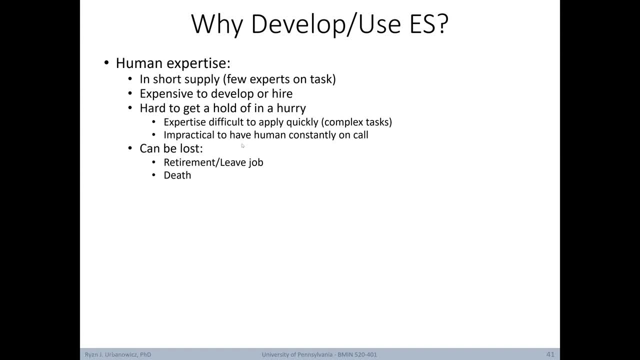 and it may take them some time to apply their knowledge. Further, it can be impractical financially to have a human constantly on call to be able to provide their expertise. Beyond this, experts can be lost due to retirement, leaving their job or death. 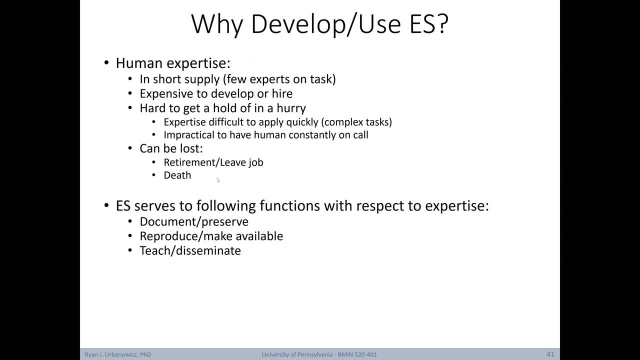 Implicitly. expert systems serve the following functions with respect to expertise. when they're developed, They can serve to document or preserve expertise, to reproduce or make available that expertise on demand, and they can be used to teach or disseminate expertise that's been stored as part of that expert system. 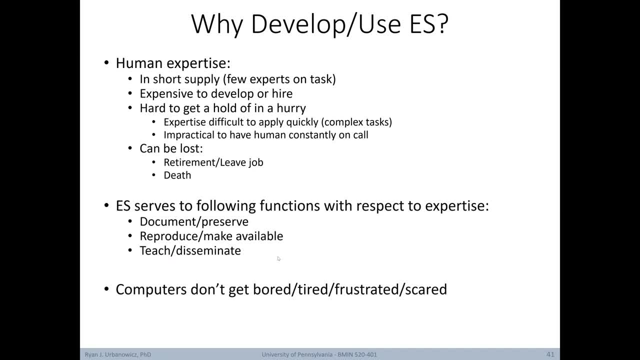 Beyond all of this, at the end of the day, computers don't get bored, tired, frustrated or scared, So having distilled human expertise into a computational form avoids some of these issues as well. In terms of their application, there are many broad classes of expert systems. 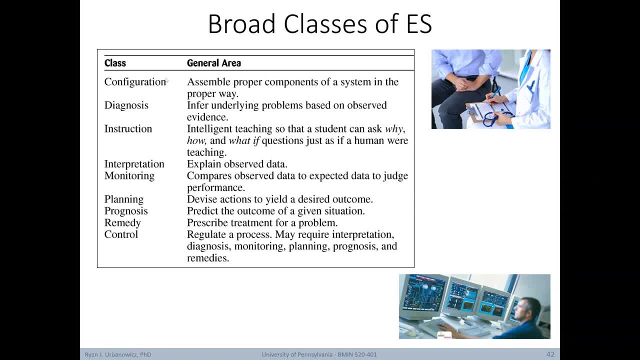 They've been designed to handle configuration problems, in other words to assemble proper components of a system in the proper way. They've been applied to diagnosis, in other words to infer underlying problems based on the observed evidence. Also to instruction, Thanks to their justification systems. 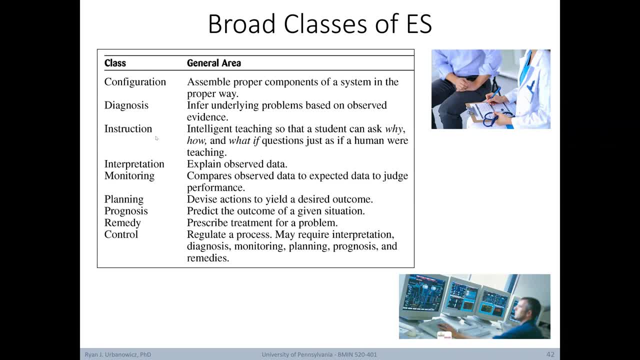 they can provide intelligent teaching so a student can ask why, how or what if questions, just as if a human being were teaching. They can also be applied to interpretation problems, where we want to explain observed data. monitoring, where we want to compare observed data. 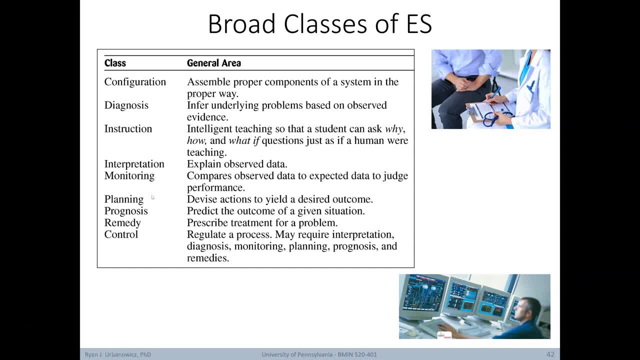 to some expected data and judge performance. also, planning, where we want to devise actions to yield some desired outcome. prognosis, where we want to predict the outcome of a situation for remedy, to prescribe treatments for a problem. and finally, control, where we might want to regulate a process. 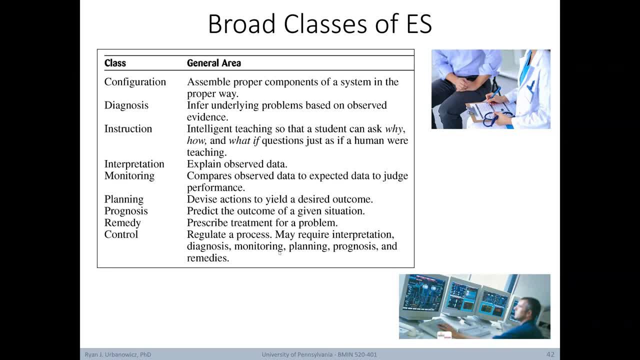 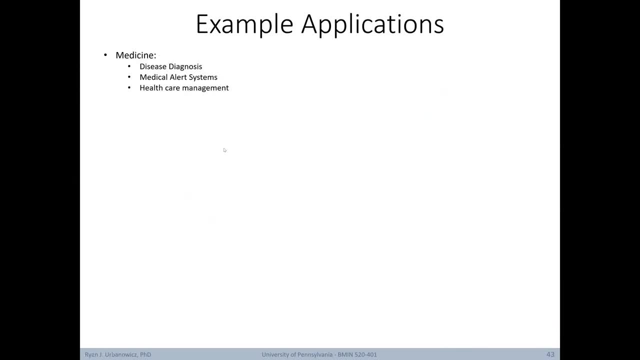 Further. a control system might also require interpretation, diagnosis, monitoring, planning, prognosis and remedies, all achieved by one single system. Here are some examples of some specific areas where expert systems have been used In medicine. we have disease diagnosis, medical alert systems. 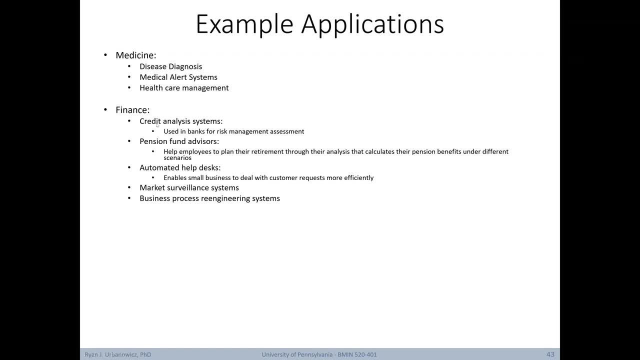 and healthcare management. In finance we have credit analysis systems, pension fund advisors, automated help desks, market surveillance systems and business process reengineering systems. In manufacturing we have machine fault diagnosis, robotics, computer configuration and material spillage identification. 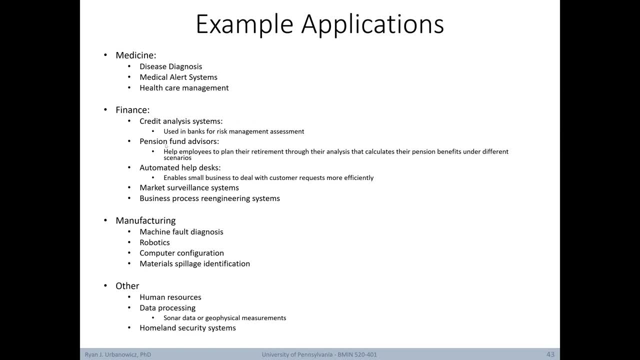 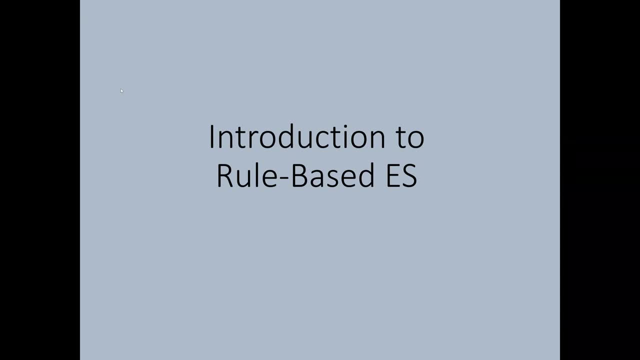 And beyond that, we've seen them used in human resources, data processing and homeland security systems. As a segue into our next lecture, we're now going to give a brief introduction to rule-based expert systems. First off, recall the rule basics. 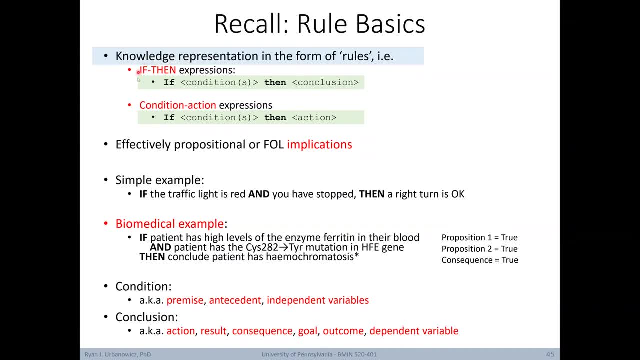 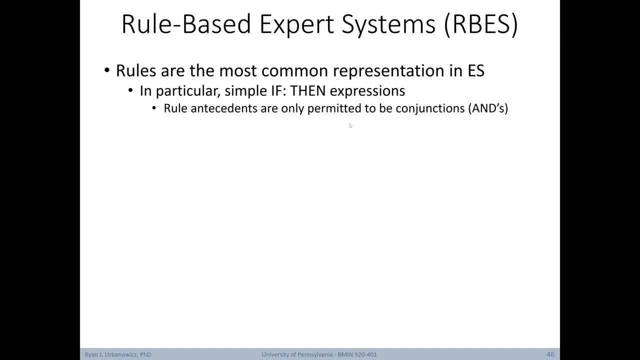 that we covered at the beginning of this lecture. In particular, we have rules given as if-then expressions. Rules themselves as a knowledge representation are the most common representation used in expert systems, In particular rules of the if-then form In such systems. rule antecedents. 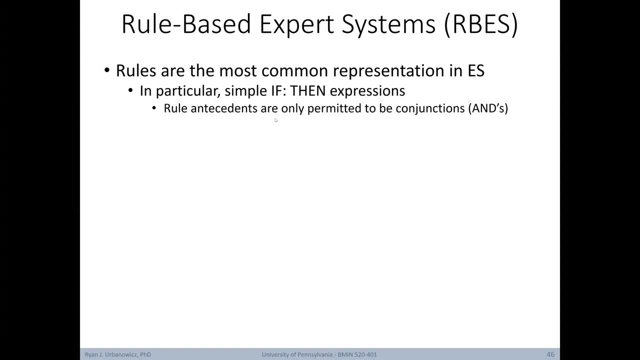 are only permitted to be conjunctions or ands. The inference engine in rule-based expert systems determines which rule antecedents are satisfied. In other words, the left-hand side must match a fact in the knowledge base. Assuming we're doing forward chaining. 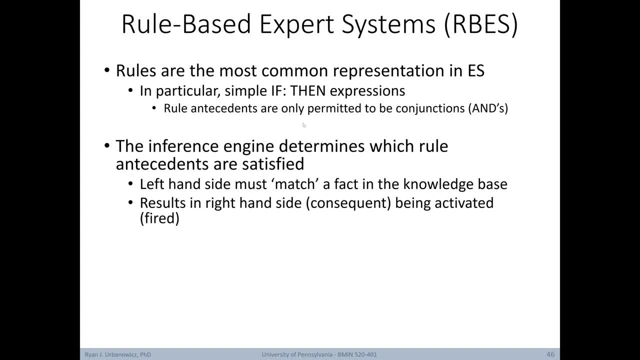 as we'll see a little bit later. When this happens, the right-hand side of the rule or the consequent gets activated or fired. This consequent activation can lead to new facts being added to the temporary knowledge base of an expert system. 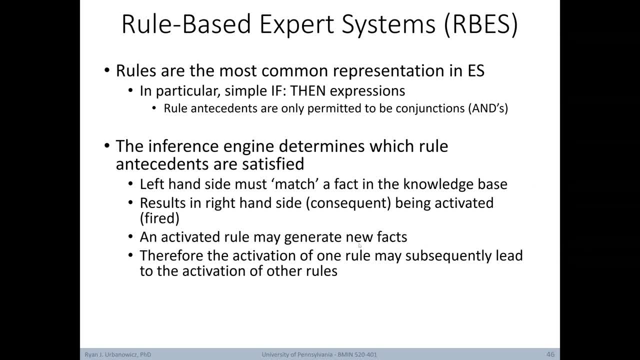 Therefore, the activation of one rule may subsequently lead to the activation of other rules downstream, once their antecedents are satisfied. For simplicity, in this course we're going to focus primarily on rule-based expert systems. So when are rule-based expert systems preferred? 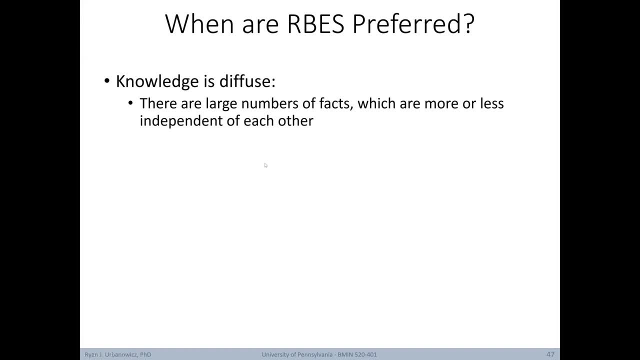 Well, first off, when knowledge is diffuse, In other words, there are a large number of facts which are more or less independent from one another. They're also preferred when knowledge can easily be separated from its use, In other words, there's no dependency. 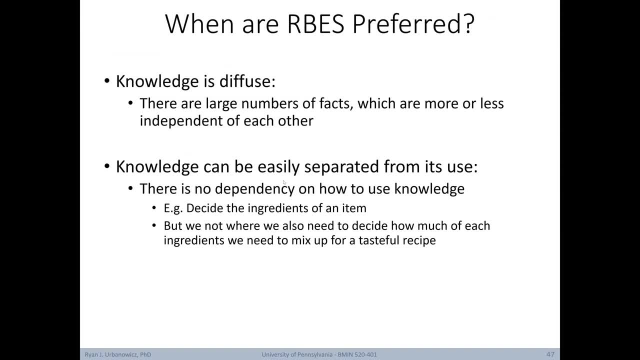 on how to use knowledge, For example, when we need to decide the ingredients of an item, but not so much when we need to decide how much of each ingredient we need to mix up together for a tasty recipe- Another term that you'll hear- that is useful. 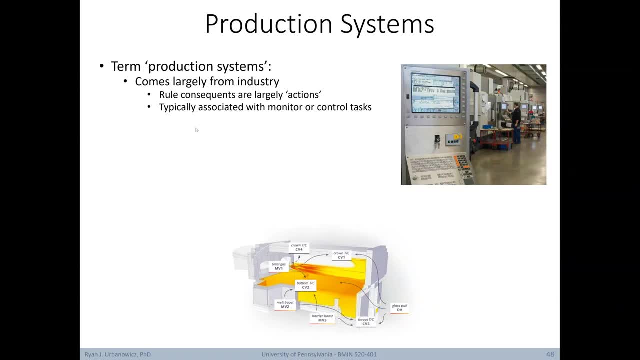 to define now is that of production systems. The term production systems comes largely from industry, And in these situations, the consequence of rules are usually actions. The term production systems is typically associated with the monitoring or controlling of tasks. However, I've noticed that there's an inconsistent 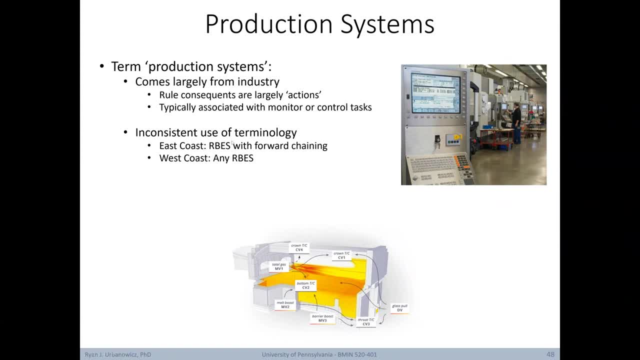 use of this terminology On the East Coast, production systems usually refers to rule-based expert systems that use forward chaining in particular, But on the West Coast the term production systems can refer to any kind of rule-based expert system. So for this course we will assume that 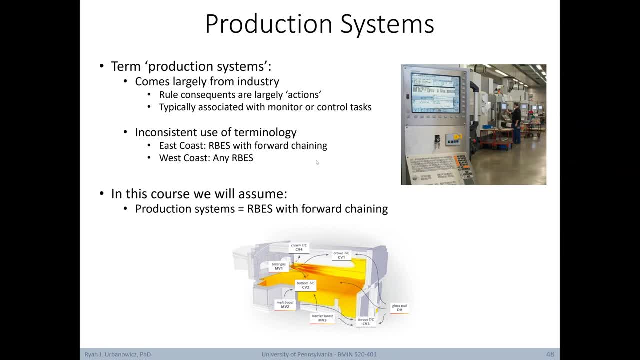 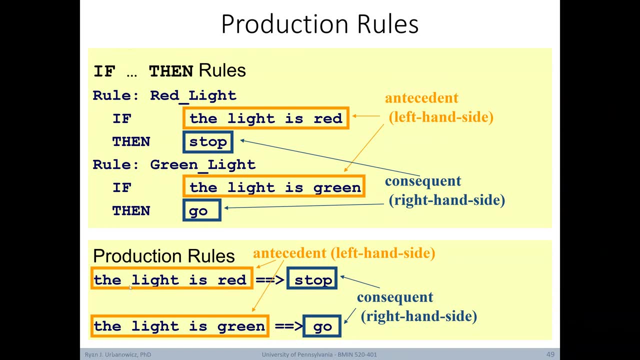 production systems refer to rule-based expert systems that utilize forward chaining. Production rules can take if-then expressions and format them in the following way. So if light is red, then stop Where we put the antecedent on the left side and the consequent on the right.